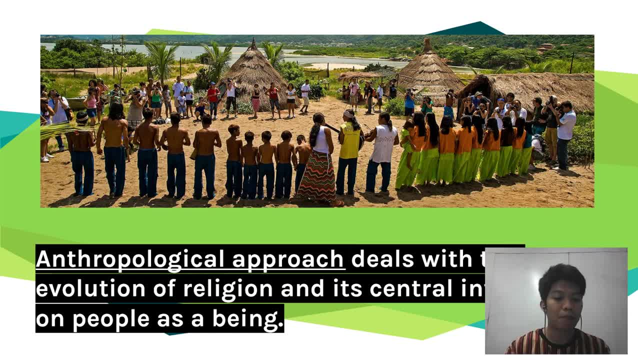 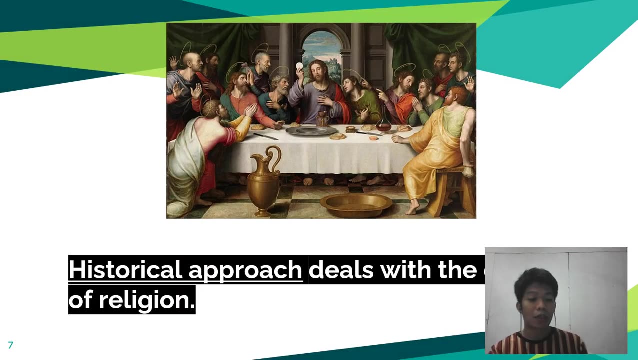 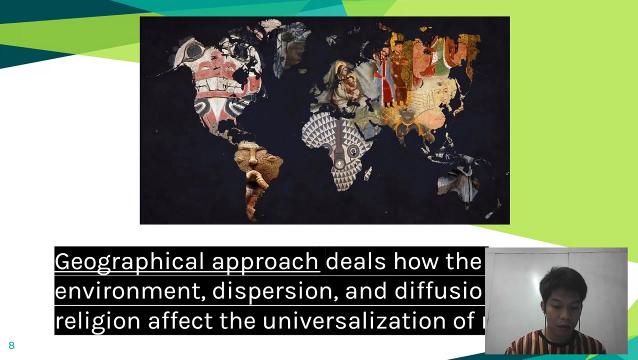 the evolution of religion and essential influence on people as a being. when we see anthropology, it is the study of society and culture and their development. in this sense, religion can influence human development as well as the society as a whole. next is historical approach: deals with the origins of religion. history is the study of 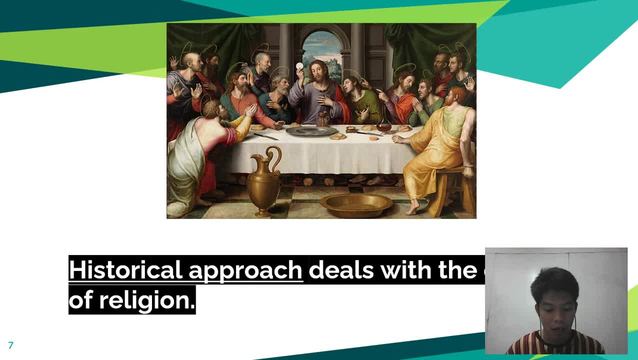 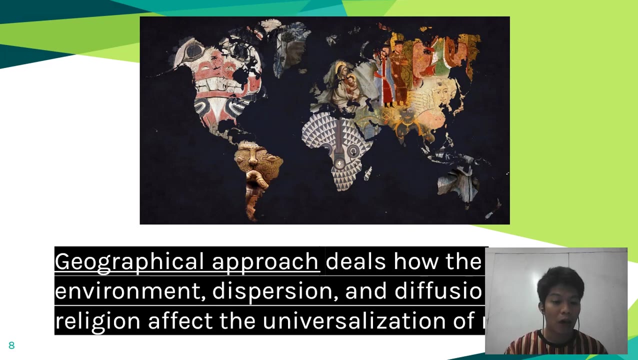 past human events. okay. thus, understanding religion in the lens of history is a way of understanding its origin. development influences from generations to generations. next is geographical approach. it deals with how the environment, dispersion and diffusion of a religion affect the universalization of religions. okay, when we say geography, it is the study of 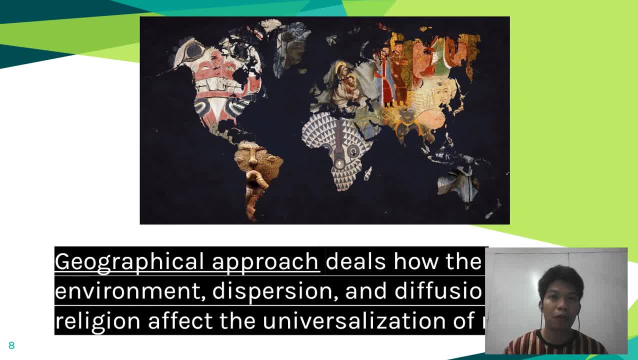 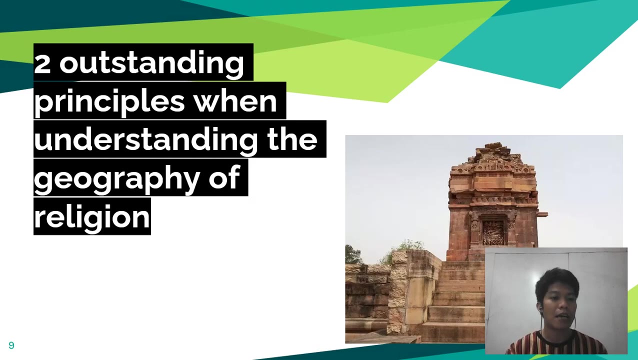 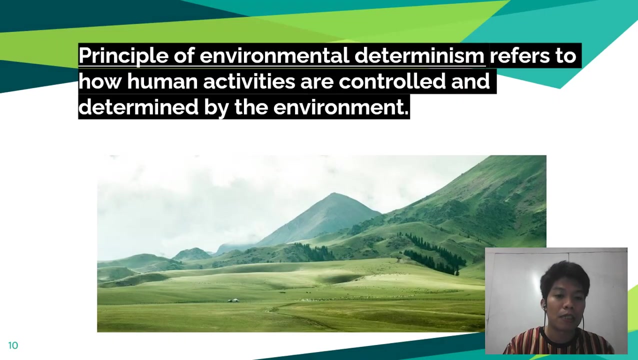 places in its relationship with people who live in a particular place. so geography can influence the origin and development of one religion. it has a big factor in how religions spread out around the world. okay, and we need to understand these two outstanding principles in understanding the geography of religion. first is principle of environmental determinism. 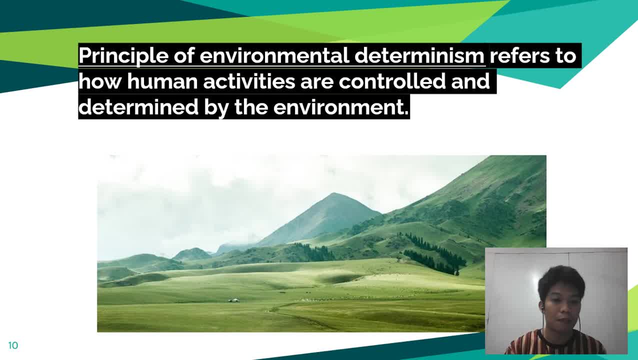 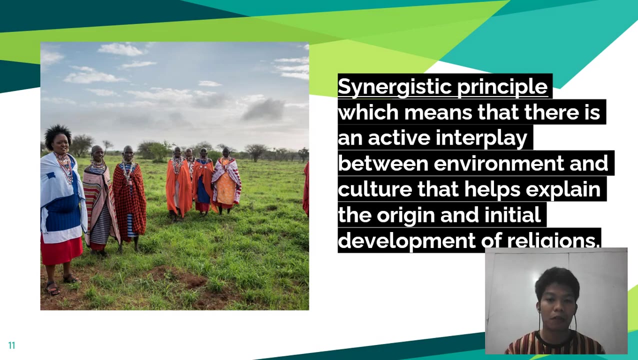 it refers to how human activities are controlled and determined by the environment. okay, when we say environmental determinism, it refers to the huge influence of physical environment to the formation of culture, religion and human activities. and we also have synergistic principle, which means that there is an active interplay between 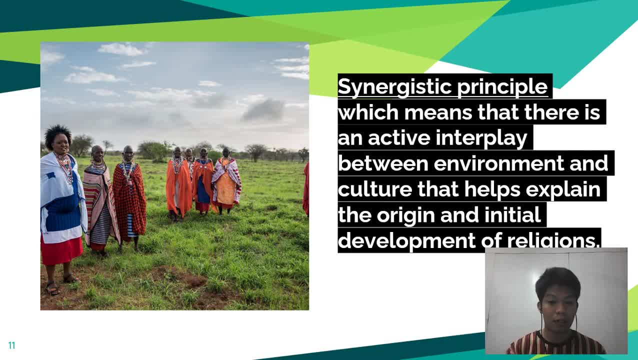 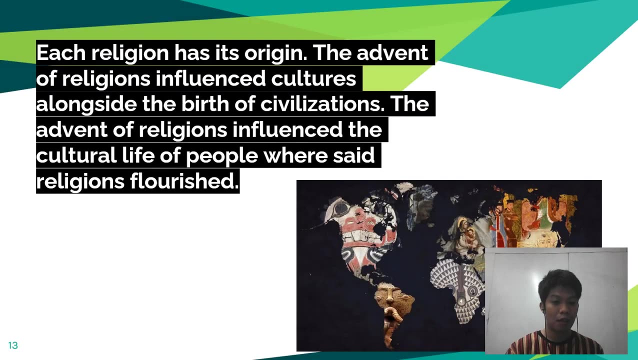 environment and culture. that helps explain the origin and initial development of religion. okay, when we say synergistic principle, it refers to the interrelatedness of environment and culture on developing a religion. next is religion and culture- okay, one of the most prominent determining factors of one religion. 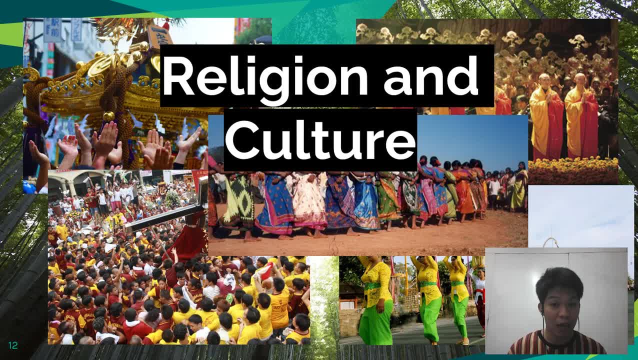 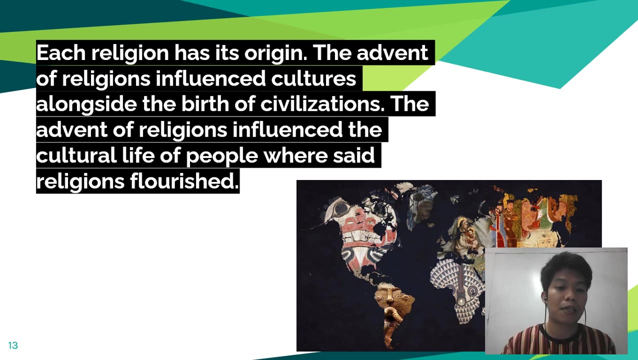 is the culture of its adherence or those who practice that specific religion. and since religion can hugely affect human behaviors and activities and it fits to study what's the effect or what's the connection between religion and culture, each religion has its origin. the advent of religions influence cultures, alongside the birth of civilizations, the advent of relations. 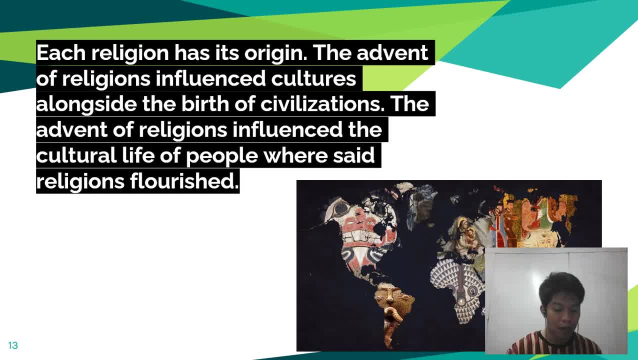 of people where said religions flourish. the religion can affect various aspects in life, and it is very evident when you look at the culture of people, in which the totality of their being and how they perceive the world are influenced by their beliefs and the system that their community has been practicing in the process of how religion creates. 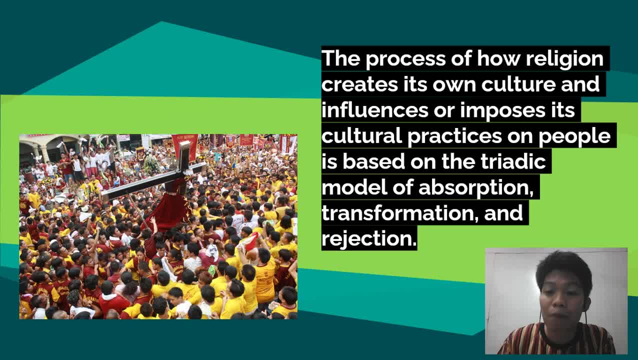 culture and influences or impulses its cultural practices and people is based on that triadic model of absorption, transformation and rejection. so these three factors- absorbed, absorption, transformation and rejection- are the manifestations of how religions evolve or spread out to various places. so when we say absorption it means 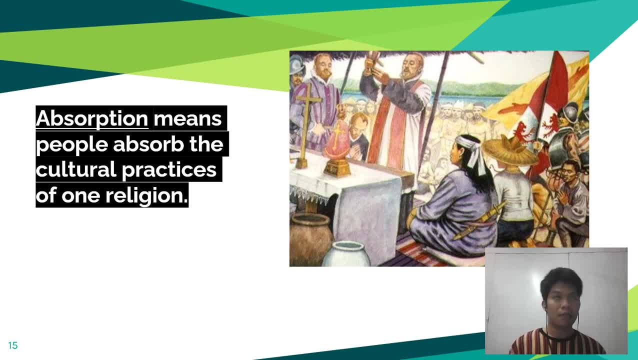 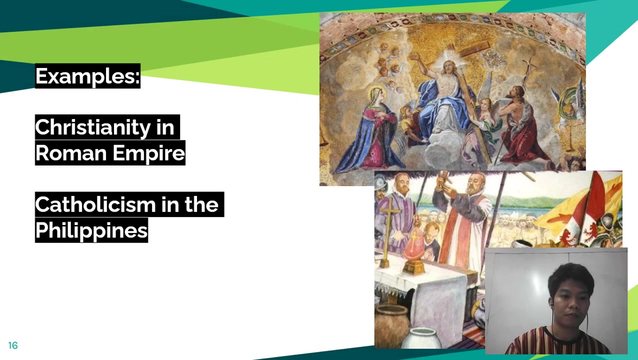 absorb the cultural practices of one religion. it means that people accept and immerse the religion being introduced to them on their own system, like, for example, the absorption of Roman Catholicism in the pre-colonial Philippines or the absorption of Christianity in ancient Rome. examples Christianity and Roman Empire and the Catholicism in the Philippines. so 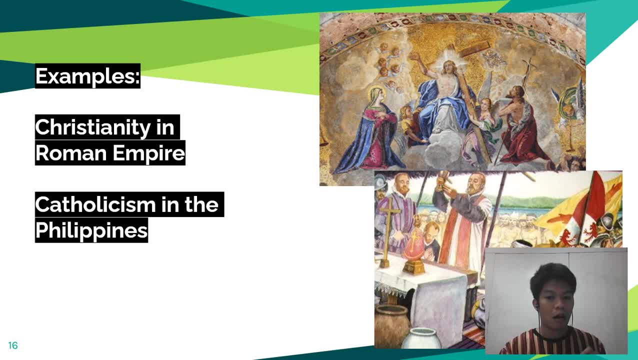 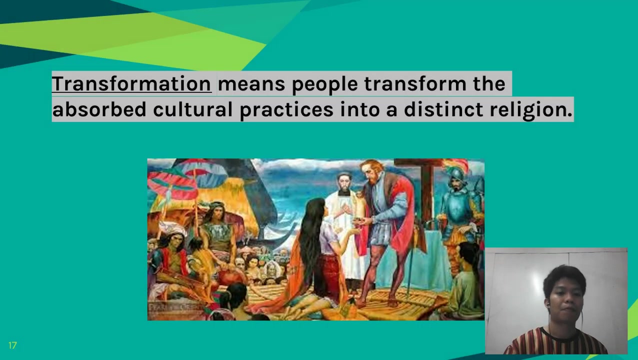 before. in the Philippines, the original religion was called as animism or anito-anito, and as well as in Roman Empire. in ancient Rome their religion was Mithraism, but then Christianity was introduced and they accepted it. next is transformation. it means people transformed, absorbed cultural practices. 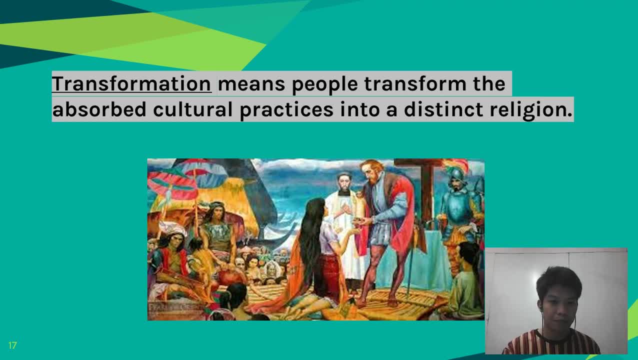 into a distinct religion. okay when we say transformation, the cultural practices and tradition of the absorbed religion transformed into a distinct variant of such religion from other adherents, especially when combining former religion. okay, for example, the absorption of Christianity in ancient Rome that practiced Mithraism. it is a pagan religion, one of the. 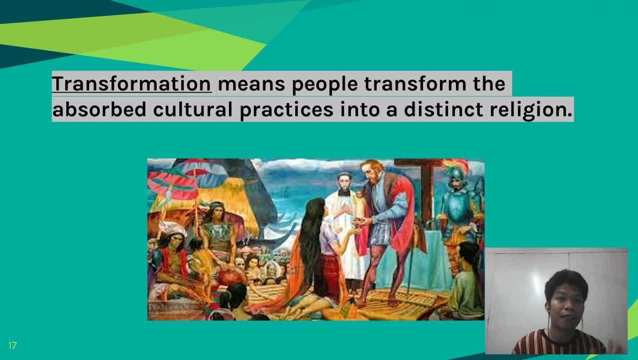 manifestations is the name of the days in calendar. for example, Sunday refers to sun, God. Monday refers to moon, god. Tuesdays refers to Seven days, because the day of Monday will be the ninth day of Ramadan. Tuesday refers to Mars, Wednesday refers to Mercury, Thursday refers to Jupiter, Friday refers to Venus and Saturday refers to Saturn. 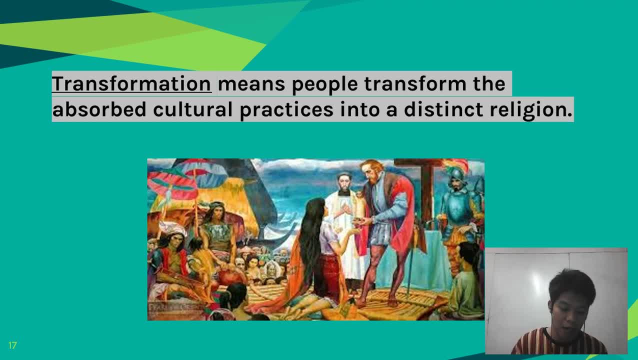 Even though Christianity believes in one God, but still their paganistic origins influence the absorbed Christianity. That's why we have what we call Roman Catholicism, because they're also distinct from other Christian religions or Christian denominations. And in the Philippines, one of the manifestations is the folk medicine. 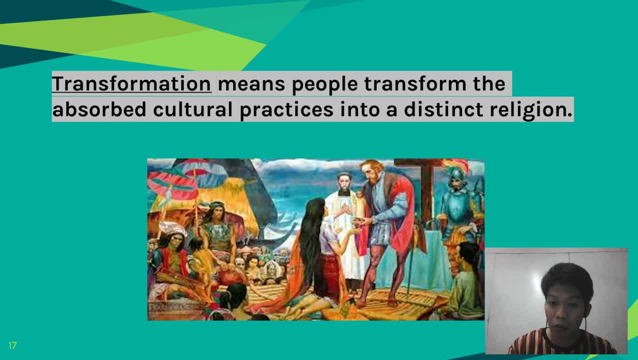 When we say folk medicine, it is practiced by quack doctors or albulario. They use medicinal plants and rituals, Influencers Influenced by animism, the original religion of the Philippines, And they also use Latin words influenced by Roman Catholicism and by calling the names of patron saints. 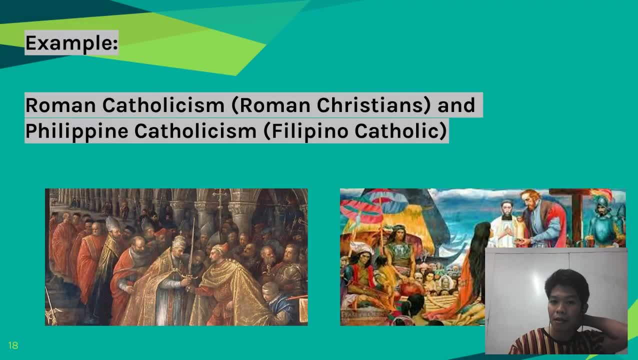 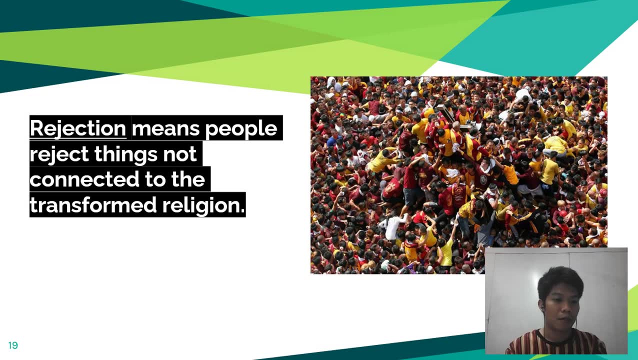 And that's it. Roman Catholicism, or Roman Christians in Philippine Catholicism are Filipino Catholic. Next one is rejection. It means people reject things not connected to them. It means people reject the transformed religion. When we say rejection, we're rejecting some of the beliefs of the absorbed religion, when it is not relevant to their original beliefs and practices. 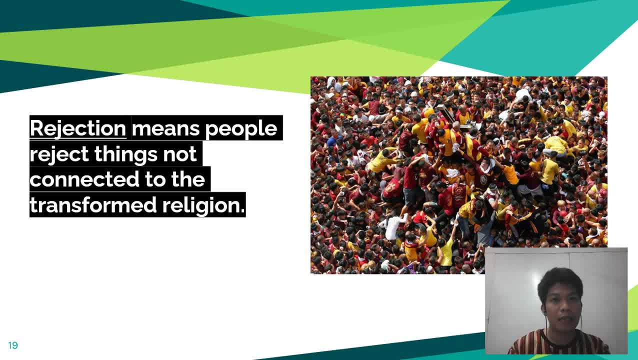 For example, in Roman Catholicism they rejected the idea that priests can marry and have a family of their own, Because in biblical times the priests or the Levites were allowed to marry, But in Roman Catholicism priests are not allowed. 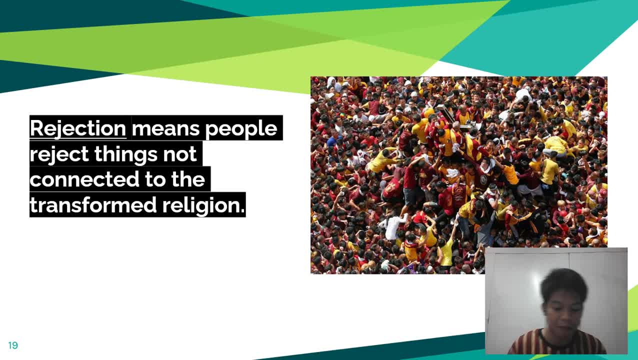 In Filipino Catholicism. they rejected the Holy Spirit because they believed that the third person in Holy Trinity is God. Is God the Mother, Since there is God the Father and God the Son. Filipino Catholicism is different from major Catholicism in the Philippines. 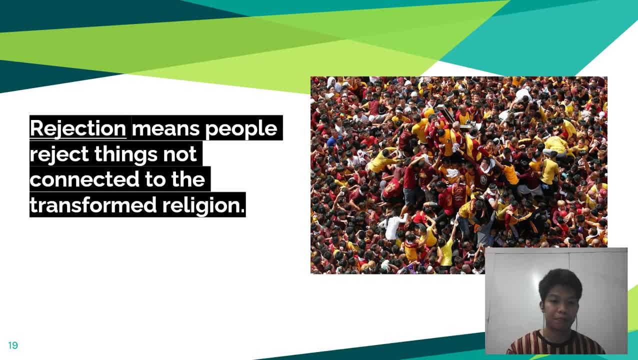 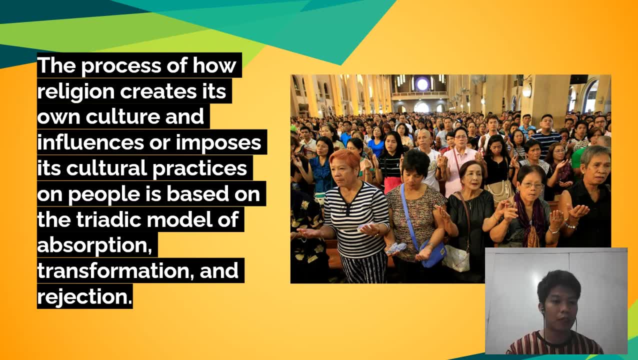 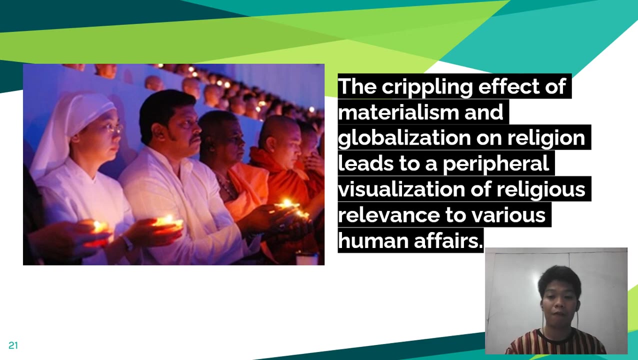 It's different. The process of how religion creates its own culture, influences or imposes its cultural practices on people is based on the tragic model of absorption, transformation and rejection. That's what we discussed earlier. The crippling effect of materialism and globalization on religion leads to a peripheral visualization of religious relevance. 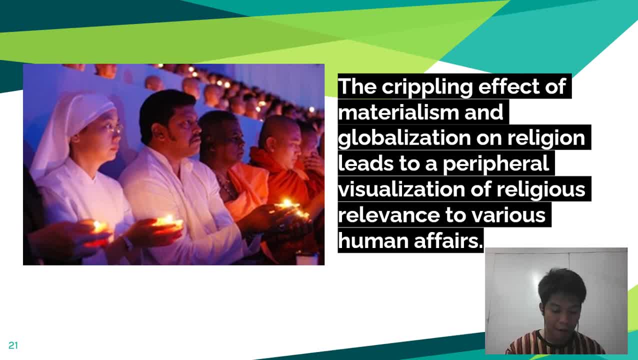 Relatives to various human affairs. In modern times, because of the advent of technology, many people are forgetting or ignoring their religious background, since their beliefs are now associated with modernity, Or, because of the modernization there's, the evolution of their beliefs and practices. 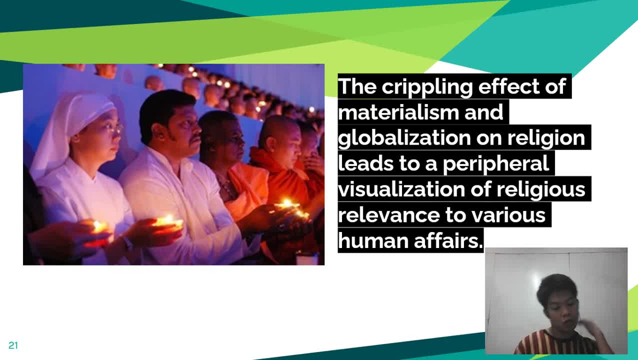 Religion can also shape their society's destiny. It also provides a template on how to manage and direct one's life. It imposes standards of what a person ought to do or not to do. In short, the moral dimension of one's actions is guided by his or her religious beliefs. 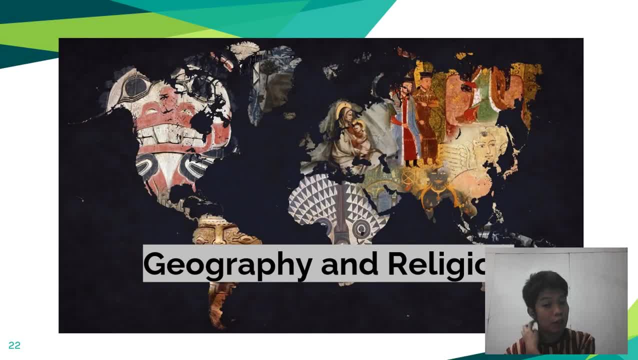 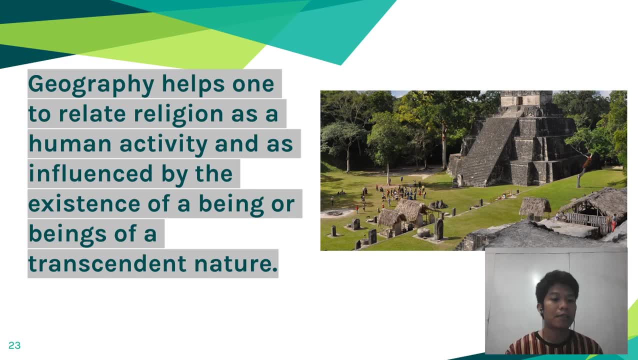 Next is geography and religion. Geography helps one to relate religion as a human activity and as influenced by the existence of a being or beings of a transcendent nature. The place and environment where people live had a huge influence to their beliefs about gods or supreme beings. 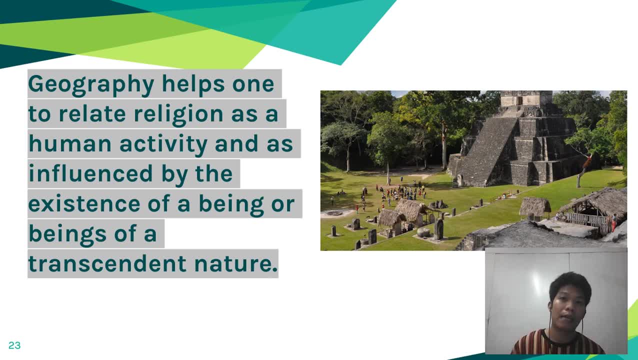 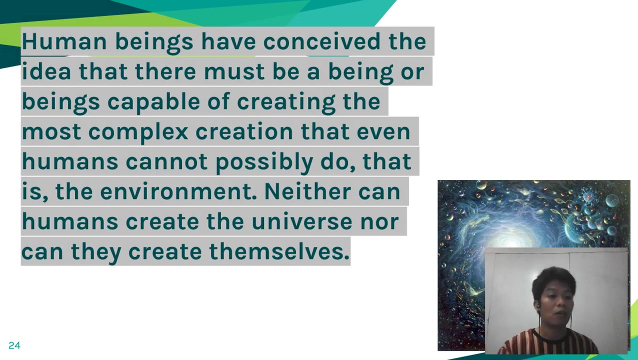 Some people worship the nature because they believe that the spirits of nature will bless their agriculture if they will worship them. Or some believe that being one with nature is a spiritual experience. Human beings have conceived the idea that there must be beings or beings capable of creating the most complex creation that even humans cannot possibly do. 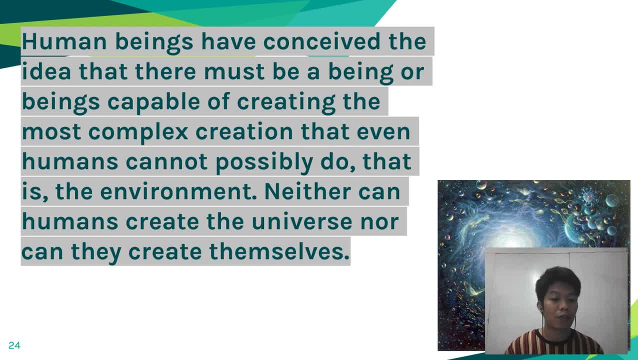 That is the environment. Neither can humans create the universe, nor they can create themselves. Nature and environment. Nature and environment conceive us powerful beings who can create the entire universe. that humans cannot do. Thus they are worthy to worship. People regarded the environment and nature as worthy of their worship because of their necessity to worship someone that is higher to them. 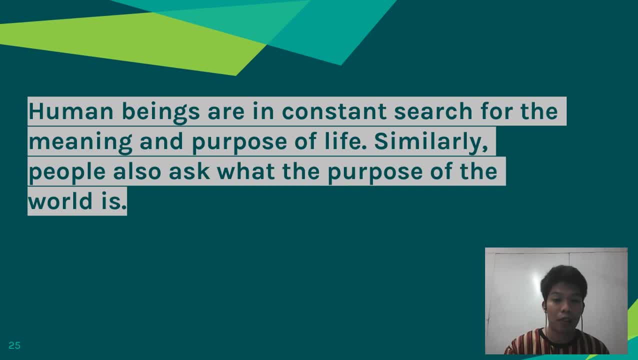 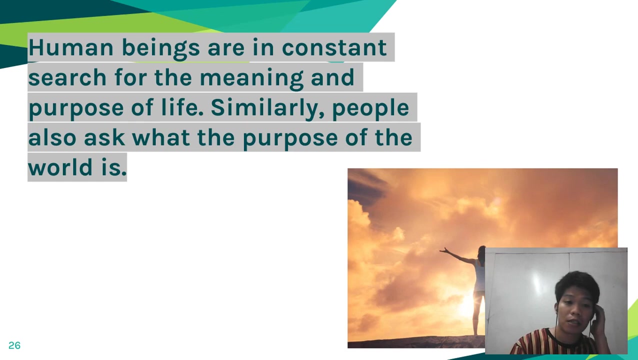 Human beings are in constant search for the meaning and purpose of life. Similarly, people also ask what the purpose of the world is. That's why people revert to the nature, because they believe that nature can give to them the purpose of their life. Human beings are in constant search for the meaning and purpose of life. 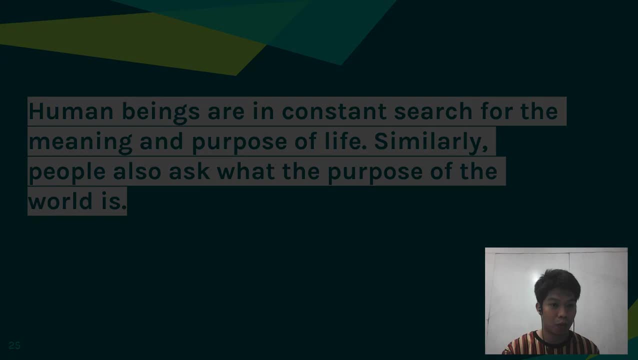 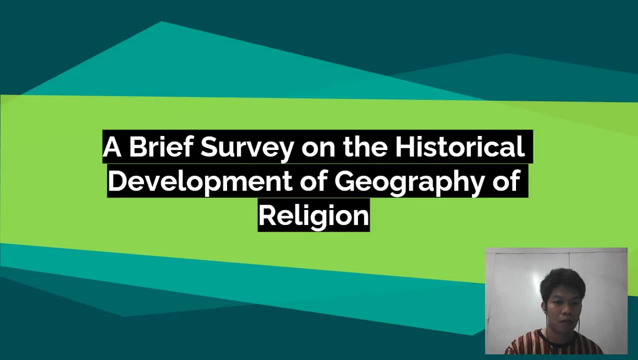 Similarly, people also ask what the purpose of the world is. That's what we discussed, That's what they help hope with. That's why people feel less, disappear from their land, Realize their time in nature and their planet, which is the basis of life. 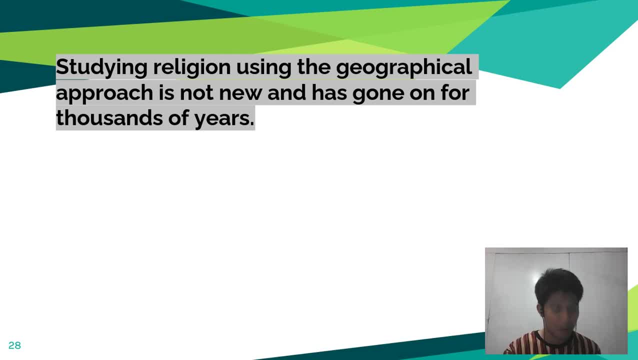 They- often guys- have had to think about what they themselves want from nature. They tend to elaborate their mechanisms in in a Lakeview area, even though it's used in nature and in a local places. Almost every local institution doing aulatorsy in every city has a lack of real political position. 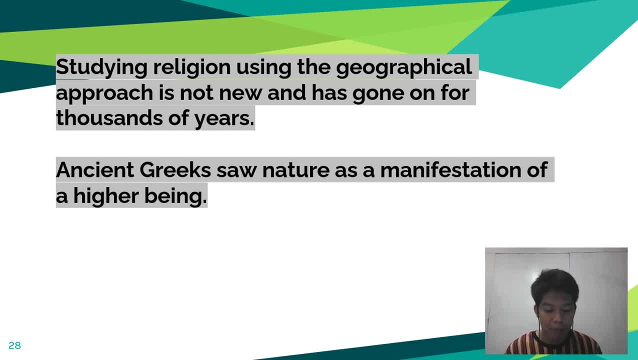 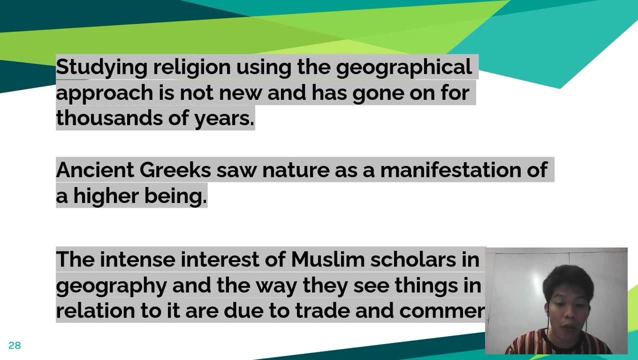 was the manifestation of supreme beings. that's why, in studying religion, was important for them to consider the geographical location of the religions. the intense interest of Muslim scholars in geography and the way they see things in relation to it are due to trade and commerce. in Islam, it spread out. 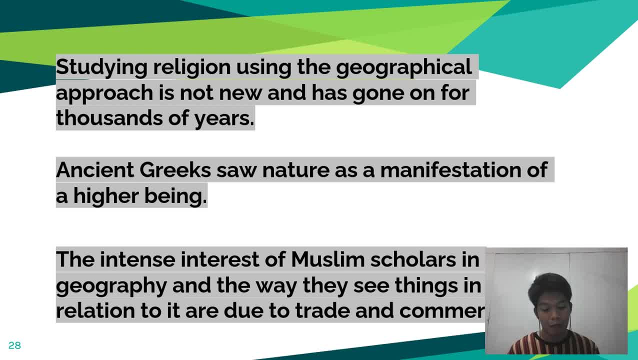 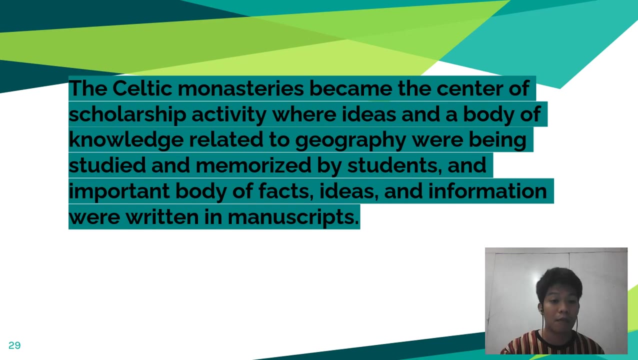 primarily because of trade in business, because of the strong ties between pre-colonial Philippines and Arabs. due to this is a trading, many parts of the Philippines converted to Islam. the Celtic monasteries became the center of scholarship activity, for ideas in a body of knowledge related to geography were being studied and memorized by 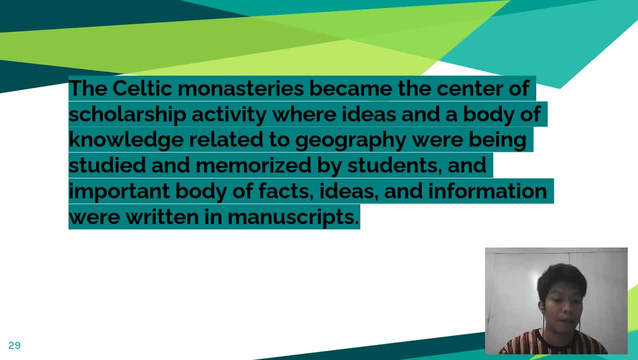 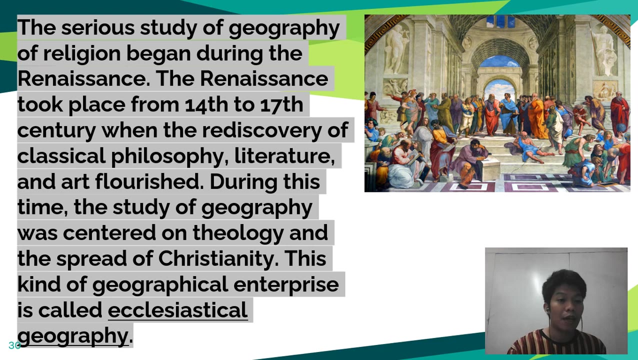 students and, importantly, body of facts, ideas, information were written and manuscripts. so even in the old times geography was widely used or widely considered as an important lens in studying religions. the serious study of geography of religion begun during the Renaissance. the Renaissance took place from 14th to 17th century, when the 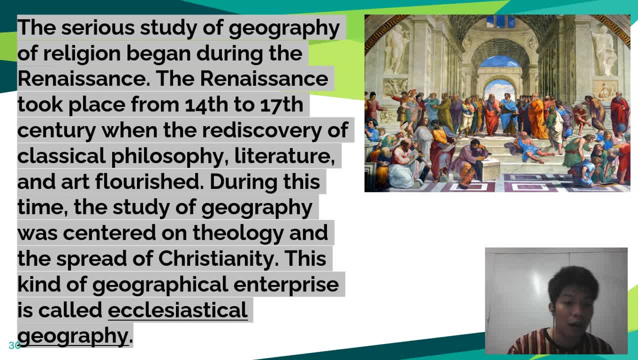 rediscovery of classical philosophy, literature and art flourished and the. during this time, study of geography was centered on theology and the spread of Christianity. this kind of geographical enterprise is called a classiestical geography, you see, Renaissance period. it is considered as the rebirth of European. 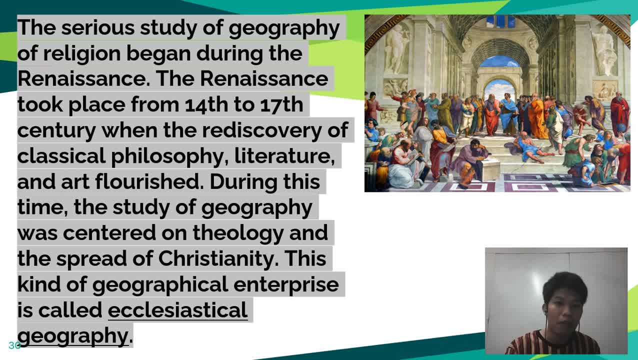 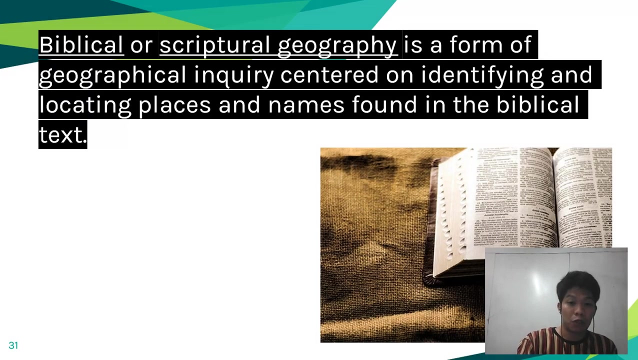 culture, politics, economics, arts and the rediscovery of classical philosophy and literature and art. so which means that equinesta ecclesiastical geography basically refers to the study of how religion of or how Christianity spread out, the relationship between Christianity and baharat. biblical or scriptural geography is it form a geographical inquiry centered on 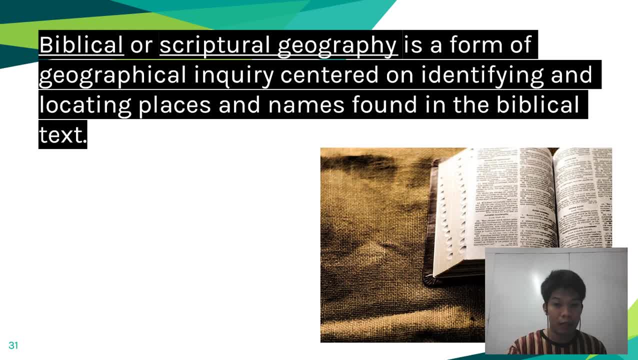 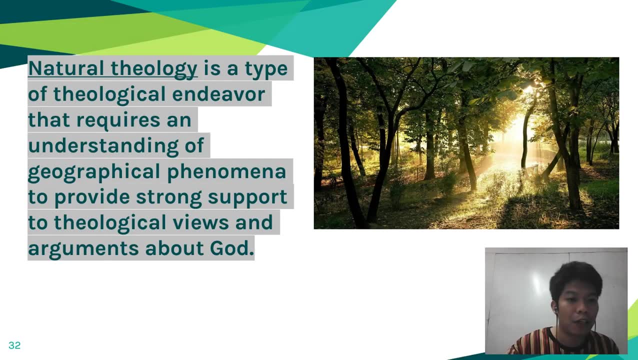 identifying and the busy places and means found in a biblical text. so biblical or or scriptural geography is finding the places mentioned in the Bible. Natural theology is a type of theological endeavor that requires an understanding of geographical phenomena to provide strong support to theological views and arguments about God. 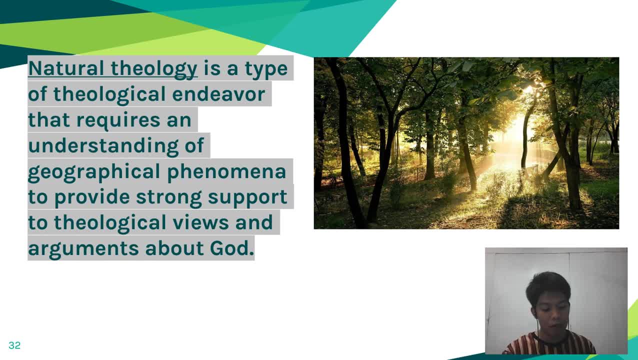 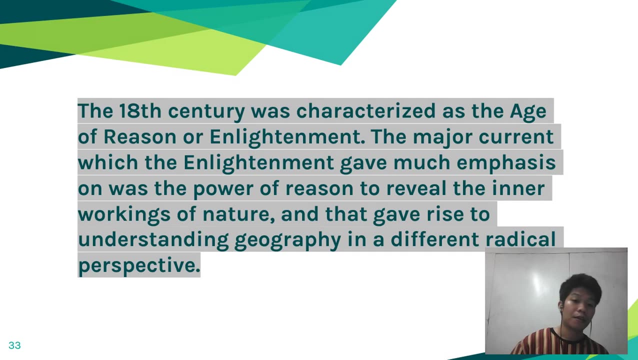 So natural. theology is the scientific or empirical aspect of explaining God in relevance to the geographical locations where events of the Bible located or events in the Bible took place. The 8th century was characterized as the age of reason or enlightenment. The major current which enlightenment gave much emphasis on was the power of reason. 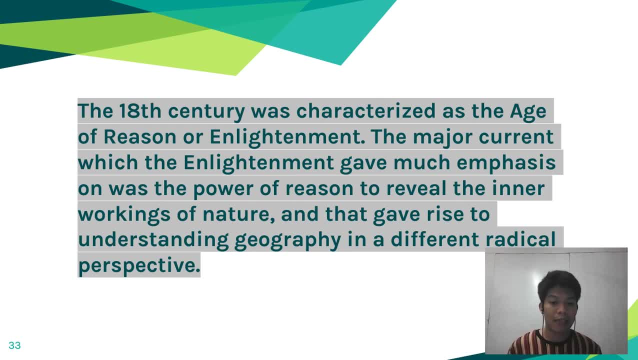 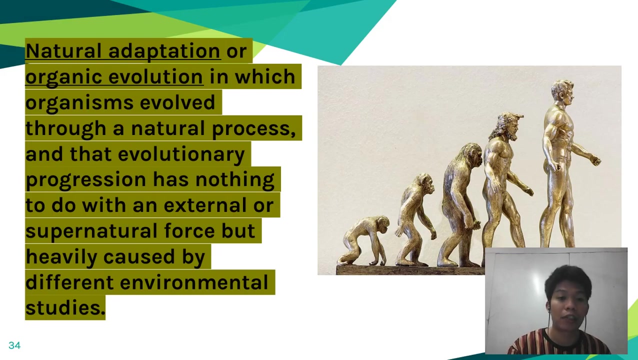 Reason to reveal the inner workings of nature and that gave rise to understanding geography and different radical perspectives. This means that logical and sound reasoning were compiled in order to explain the relevance of geography and religion during the age of reason or enlightenment. Those have natural adaptation or organic evolution in which organisms evolved. 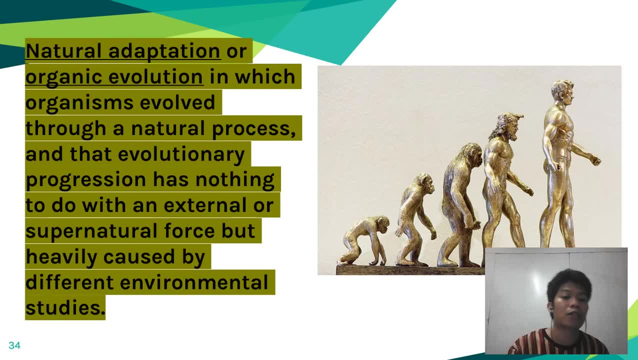 through the evolution of nature Through a natural process, and that evolutionary progression has nothing to do with an external or supernatural force, but heavily caused by different environmental studies. So environment plays or has a huge factor on the evolution of species and living things, as opposed to the divine creation most religions believe in. 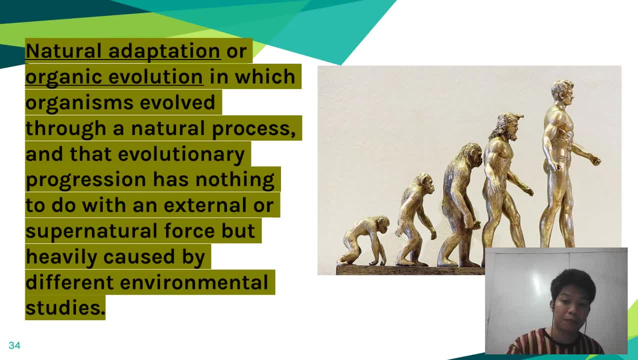 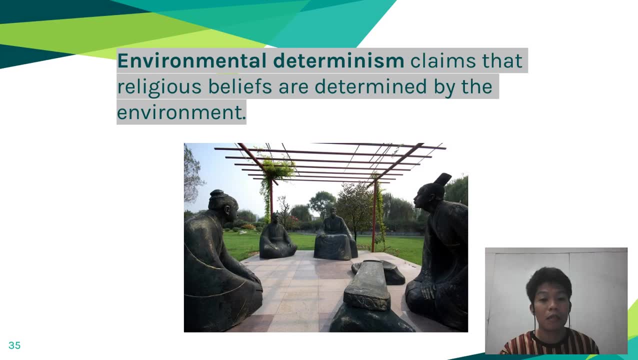 That's what we call Natural adaptation or organic evolution. We also have environmental determinism that claims that religious beliefs are determined by the environment. So the environment greatly affected the culture, traditions and beliefs valued by one religion, The fusion and dispersion of religions. 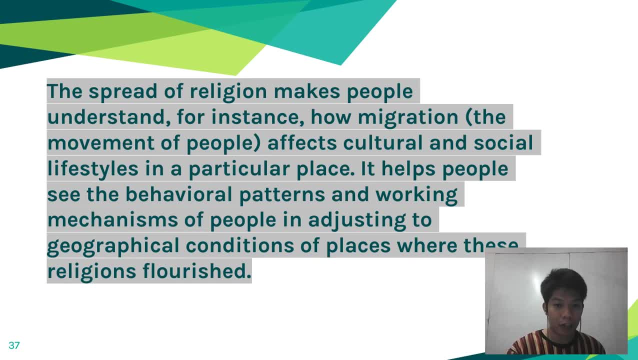 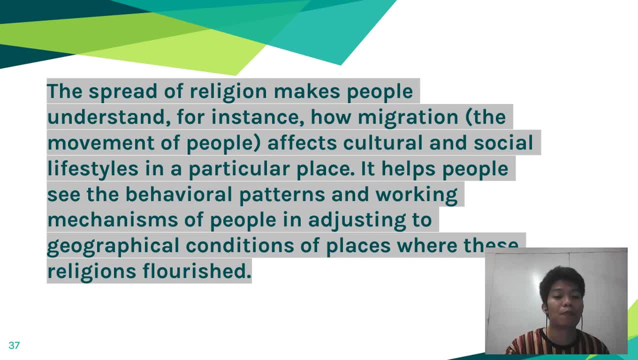 It helps people see the behavioural patterns and working mechanisms of people in adjusting to geographical conditions and places where these religions flourish. Migration is a huge factor in dispersion of religions. moving from one place to another after another affects people's culture and beliefs and even influence the people near to them, and it 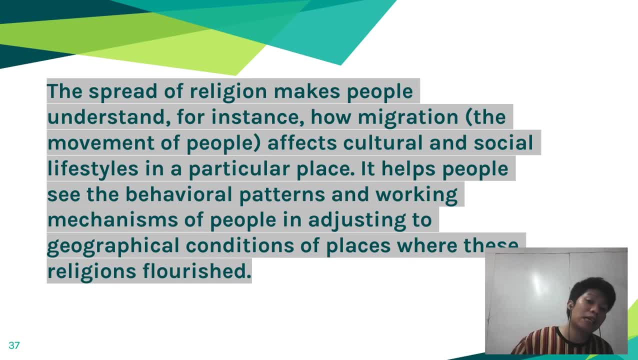 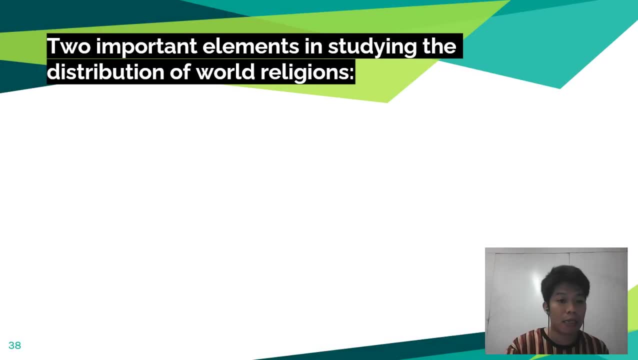 could help us grasp their way of life by seeing the patterns of their system. two important elements in studying the distribution of religions first is the places where these religions are generated. this means that we need to and to understand, we need to study where the religions come from, or their birth of origin. 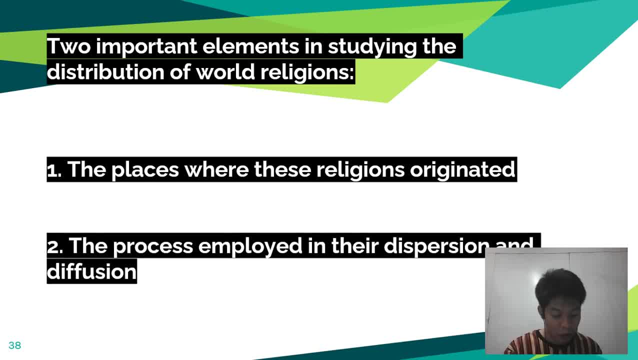 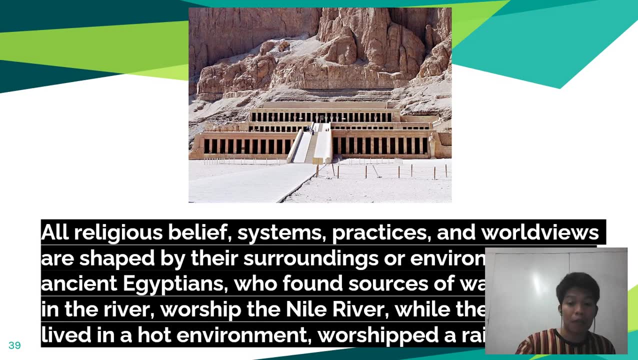 the process employed in their dispersion and diffusion, how the adherents influence other people to be accepted by other people outside of their religion. all religious beliefs, systems, practices and worldviews are shaped by their surroundings or environment. the ancient egyptians who found sources of water and food in the river worship the now river, all the hindus who 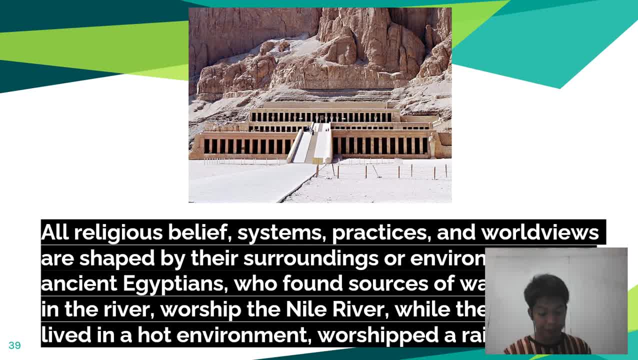 live in a hot environment. worship a rain god. the people in the ancient times usually worship the source of their food and livelihood. if, for example, the now river in egypt, because it was the main source for irrigation of their agriculture, they implored themselves to worship it. 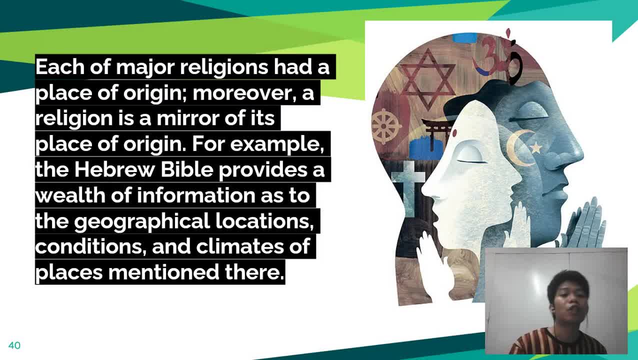 to build a new water source for irrigation for those who live in the horde. each major religions had a place of origin. moreover, a religion is a mirror of its place of origin. for example, the hebrew bible provides a wealth of information as to the geographical locations. 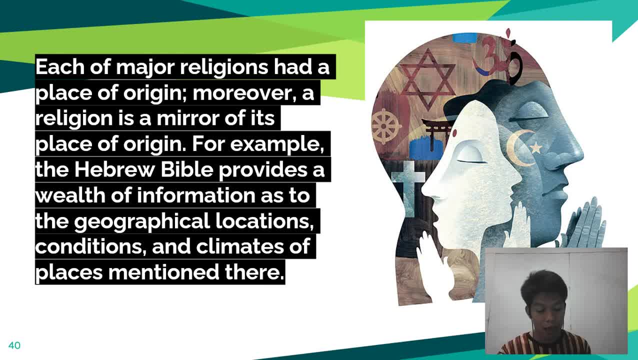 conditions and climates of places mentioned there, the place of origin, the place of origin studying religion. um, it is important to look at the place of origin and the location of religion. there is an important point here: the environment of the locations, because this will give to some important answers, explanations to. 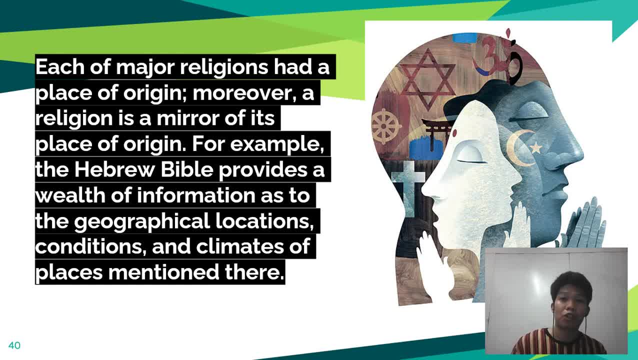 the compelling questions, because the geographical location can also affect the, the culture of the people, how they see or perceive things or the world. here, for example, in, in hebrew and jewish culture. um, they called- what do you call that the, the dead sea, as a sea where in fact, it's a form of lake, but then they called it as a dead sea. 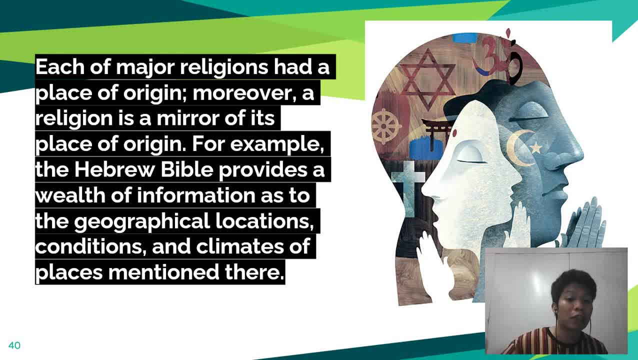 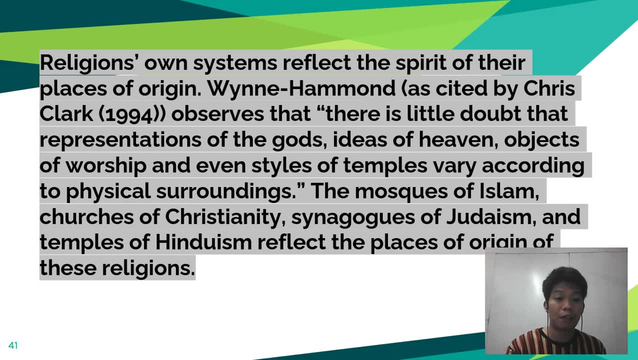 because that's how they perceive their geographical location. that's one important aspect of the differences: how we perceive our environment. religion's own systems reflect the spirit of their places of origin. wein hamann, as cited by chris club 994, observes that there is little doubt. 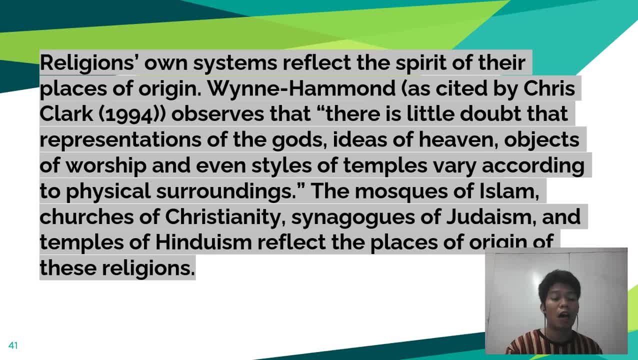 that representations of the gods, ideas of heaven, objects of worship and even styles of temples vary according to physical surroundings. the mosque of islam, churches of christianity, synagogues and temples of hinduism reflect the place places of origin of these religions. so, even though legions have variants and similarities, but the physical environment is truly manifested. 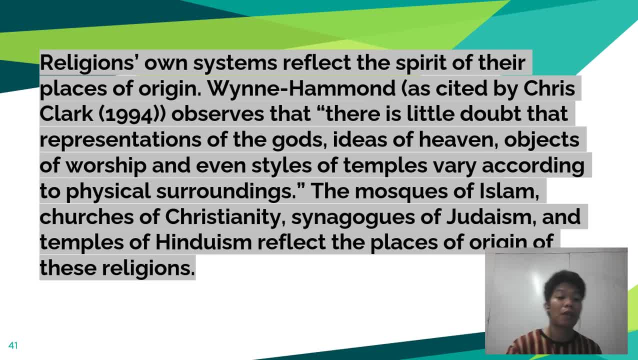 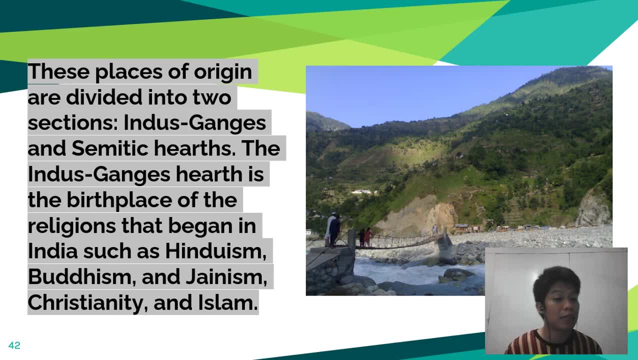 on the different styles and designs of temples and churches. these places of origin are divided into two sections in this: gangas and semitic hearts. theよろas ganga's heart is a birthplace of the religions that it began as intentioned: Perquèive, bizarreếchis and seminary obligations to be taunted for profits- a meaning that emails the Student's gave him. 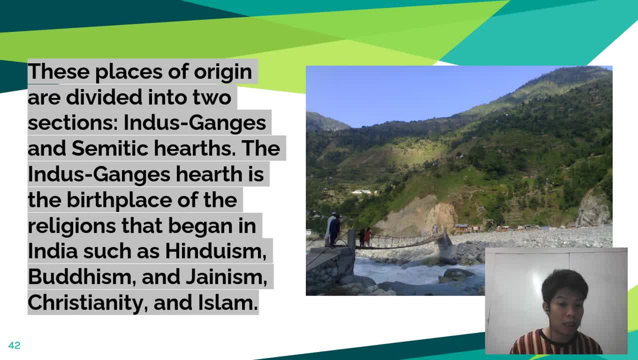 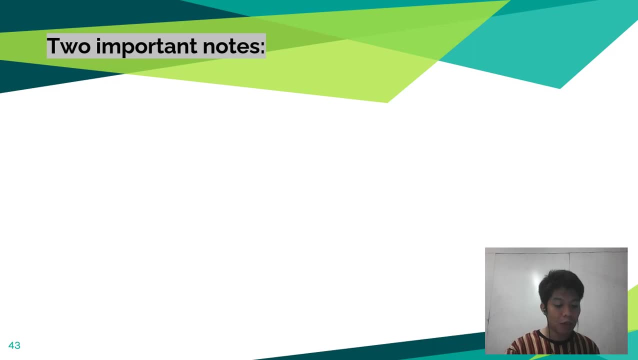 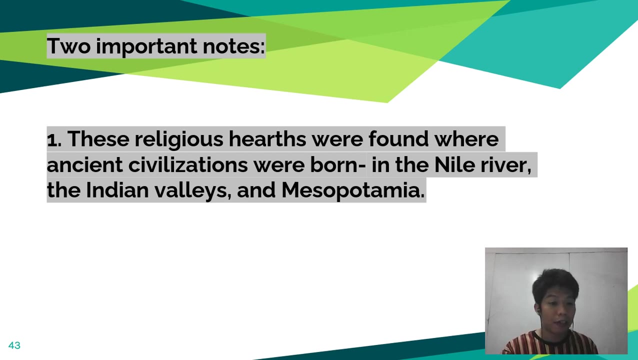 in India, such as Hinduism, Buddhism and Jainism, Semitic hearts, Christianity and Islam. It's in the Fertile Crescent. Two important notes. These religious hearts were found where ancient civilizations were born: In the Nile River, the Indian Valleys and Mesopotamia. 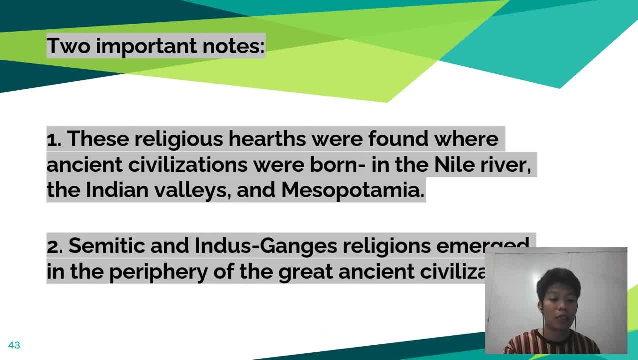 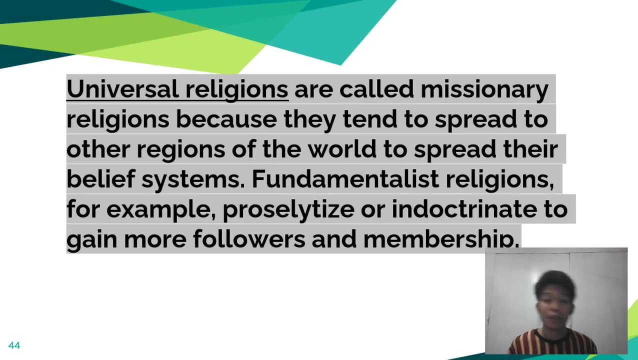 Semitic and Indus Gangas religions emerged in the periphery of the great ancient civilizations, So the birth of these religions also birthed some of the ancient civilizations in the world. Universal religions are called missionary religions because they tend to spread to other religions of the world. 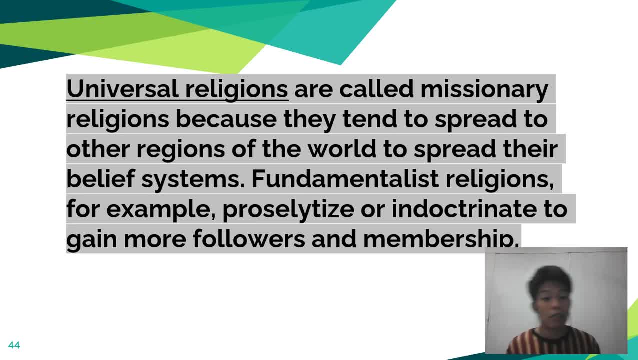 To spread their belief systems- Fundamentalist religions, for example, To proselytize or indoctrinate, to gain more followers and membership. So it is the intentional act of spreading religion, like attracting converts in order to widen their religion, To gather more members of their religion. 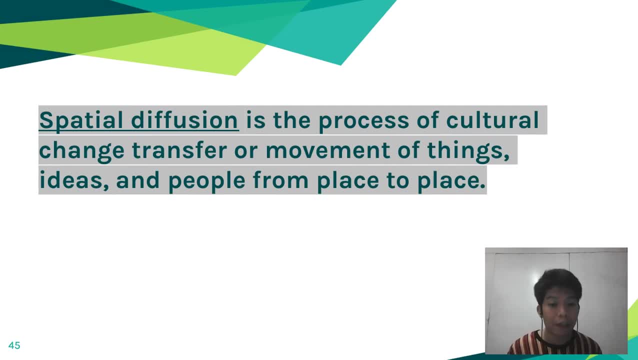 Spatial definition is the process of cultural change, transfer or movement of things, Ie to send people from place to place, Just like in Islam. the belief in Allah is not just the primary purpose of spreading Islam, But as well as their culture, their beliefs and practices. 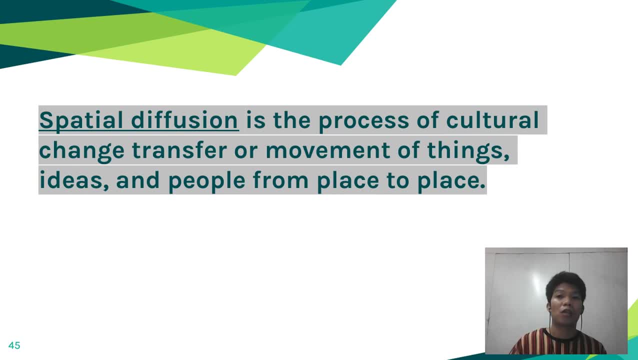 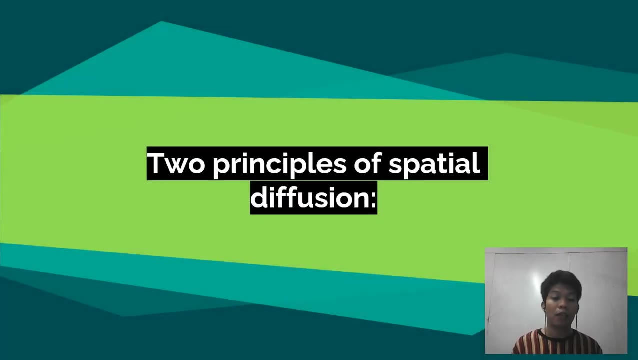 Which means that it is not just a belief that people transfer to other people, But as well as their culture, their traditions, even their rituals. And it is not just the belief that one can enter into the world without understanding the religious principles, Two principles of spatial definition: 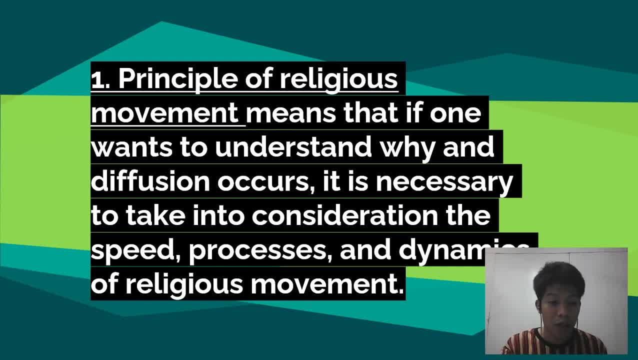 First is principle of religious movement Means that if one wants to understand why a definition occurs, it is necessary to take into consideration speed, processes and dynamics of religious movement, Which means that you need consider how fast, what's the method and the characteristic of diffusion. 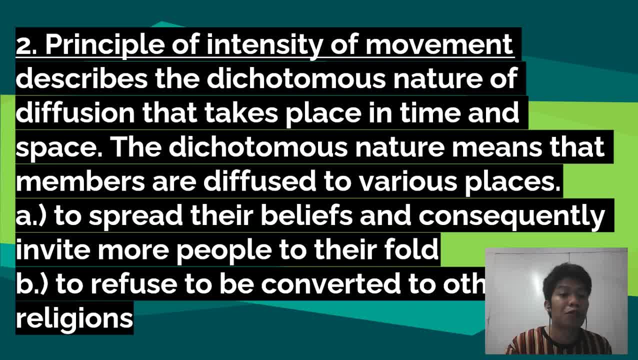 The principle of intensity of movement describes the dichotomous nature of division that takes place in time and space. The dichotomous nature means that members are refused to bar spaces to spread their beliefs and consequently invite more people to their fold and to refuse to be converted to other religions. 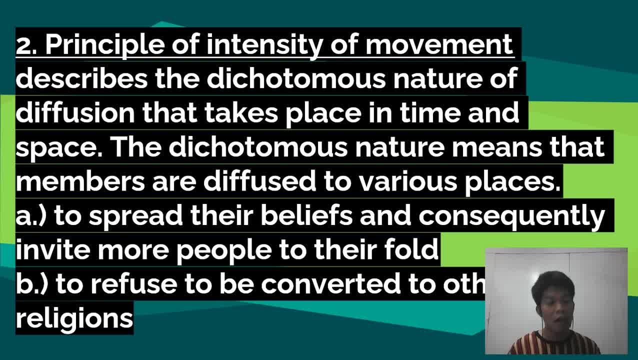 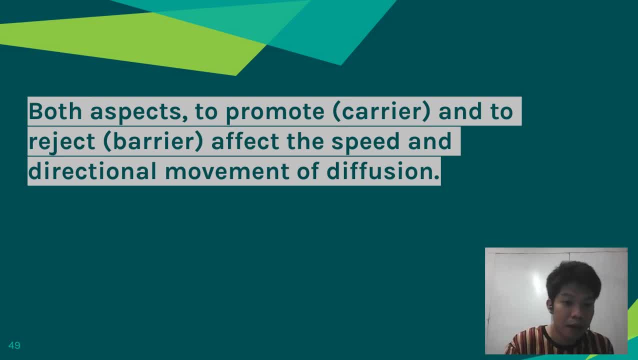 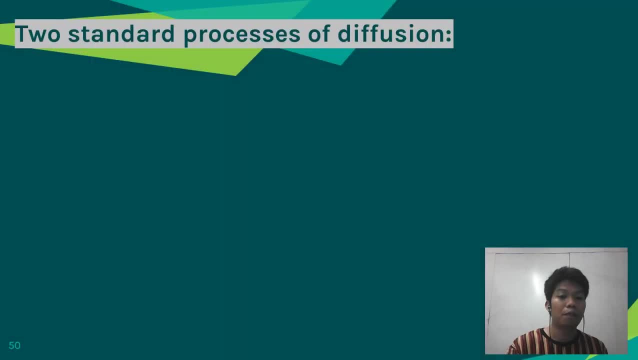 So this means that converting people to their religion, but rejecting other religions to influence them or get converted to them. Both aspects- to promote, to carry and to reject or barrier- affect the speed and direction of movement of division. So two standard processes of division. 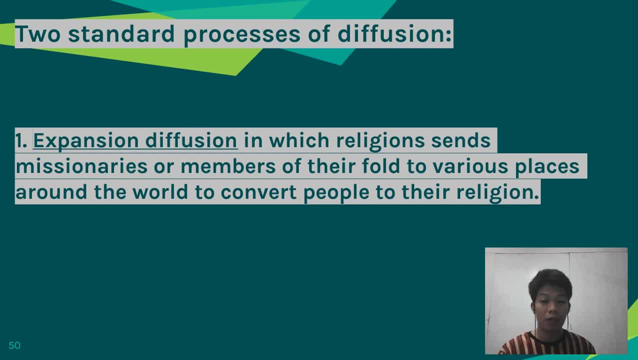 Expansion-diffusion, in which religions- Religions send missionaries or members of their fold to bar spaces around the world to convert people to their religion, Which means that sending off missionaries to spread their religion, For example, the Christian missionaries, what they did in the Philippines. 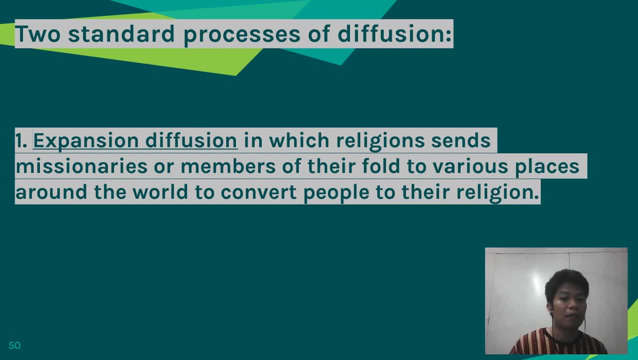 They suggest they colonize our land, but they also influence us. their religion. They subjugated our culture before they came, as well as our religious belief system. They introduced Christianity to us. That's an example of expansion-diffusion. 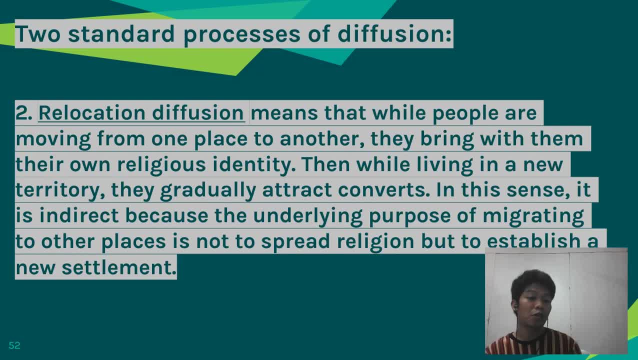 Just like this one. Next is relocation-of-diffusion. It means that while people are moving from one place to another, they bring with them their own religious identity. Then, while living in a new territory, they bring with them their own religious identity. 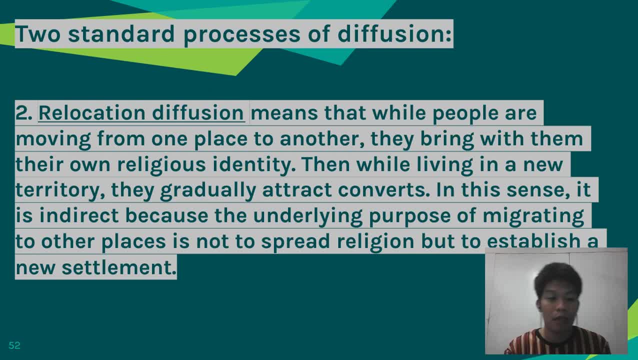 Then, while living in a new territory, they gradually attract converts. In this sense, it is indirect, because the underlying purpose of migrating to other places is not to spread religion, but to establish a new settlement. Migration is what we have discussed earlier. 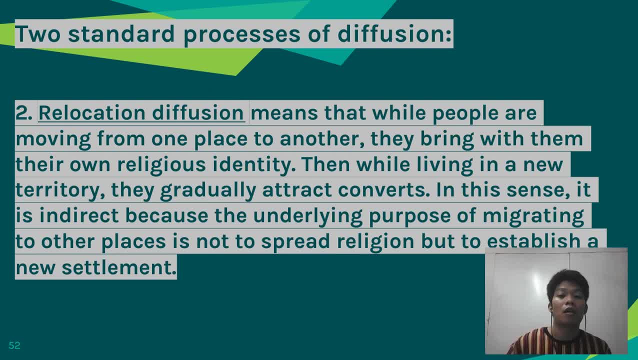 That it is one of the ways to spread one religion. When people migrate or move from one place to another, Living from one place to another, we bring their religion and influence the people who live in the community where they transferred. That's relocation-of-diffusion. 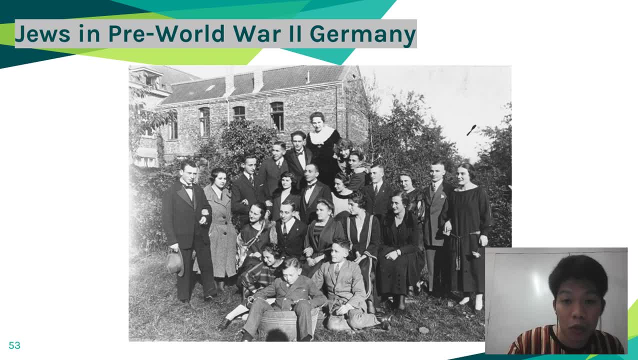 For example, we choose and bring World War II Germany Because the Jewish were spread out for many times. They spread out around the world. They brought their religion, their traditions, their practices to the place where they relocated, For example in Germany before World War II. 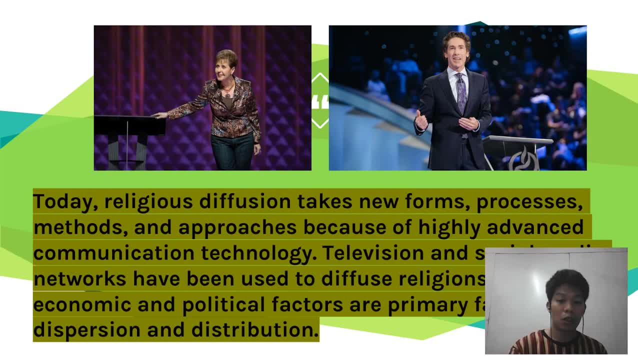 Today, religious diffusion takes few forms, processes, methods and approaches. because of highly advanced communication technology, Television and social media networks have been used to diffuse religion. While economic and political factors are primary factors of dispersion and distribution, So technology can be used to spread religion. 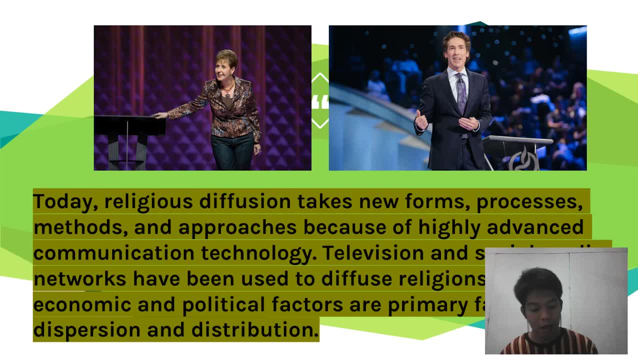 And other faiths. There are churches and denominations, Facebook fan page, Television network, Radio programs, YouTube channels And other platforms, So select this one: Joel Osten and Joyce Mayers. They have television programs. They have church services and preachings. 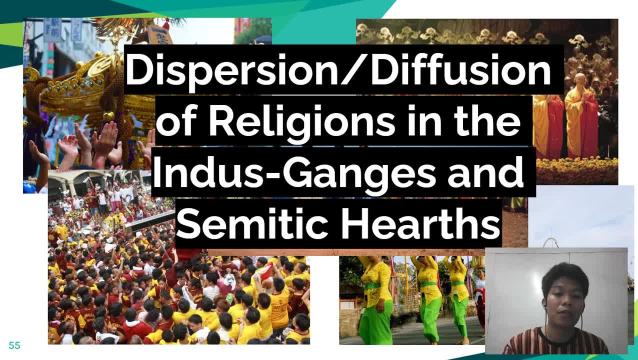 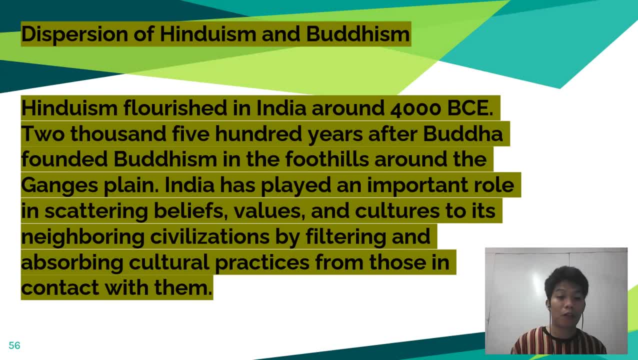 Dispersion or diffusion of religions in the Hindus, Ghanas and Semitic hearts. Dispersion of Hinduism and Buddhism. Hinduism flourished in India around 4000 BCE, 2500 years after Buddha founded Buddhism and the foothills around the Ghanas. 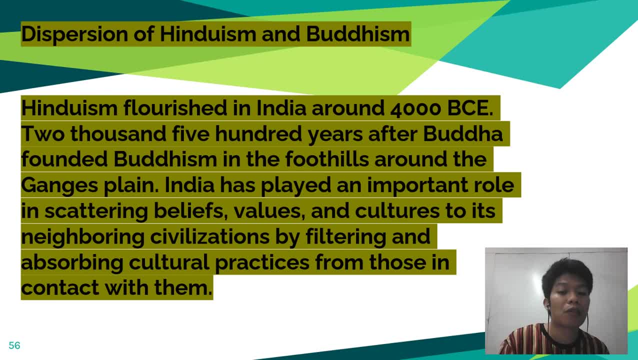 India has played an important role in scattering beliefs, values and cultures to its neighboring civilizations, by filtering and absorbing cultural practices from those in contact with them. So Hinduism and Buddhism originated from India, And by that it spread out to other regions. 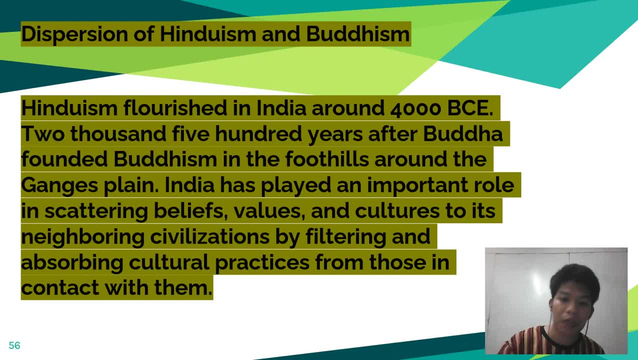 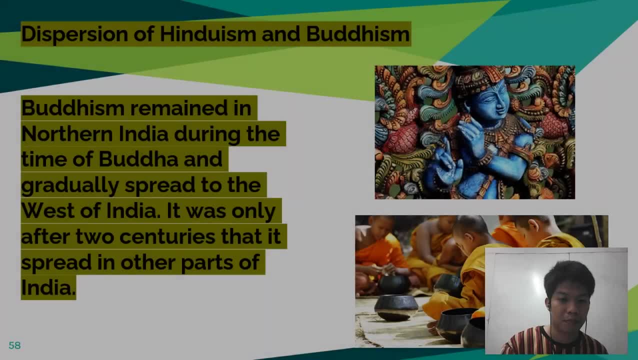 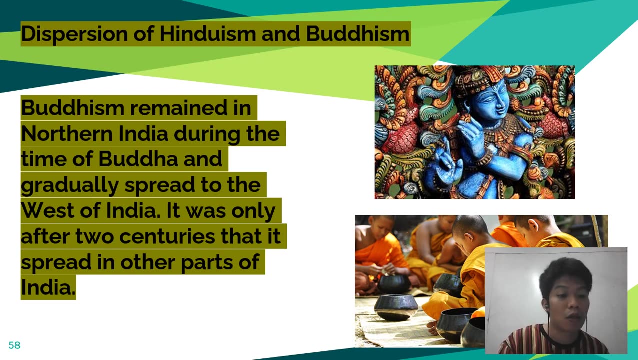 Nearby places or countries. This is the map. Buddhism remained in northern India during the time of Buddha and gradually spread to the west of India. It was only after two centuries that it spread in other parts of India, So even other parts of Southeast Asia. 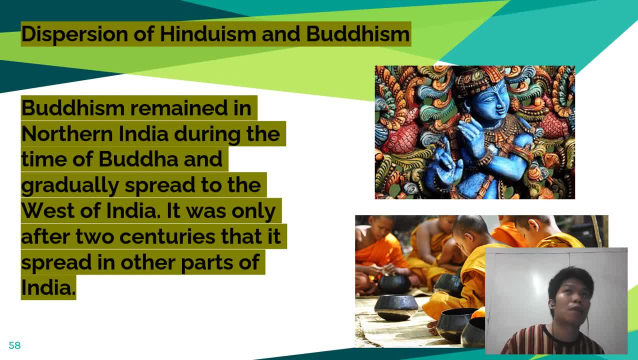 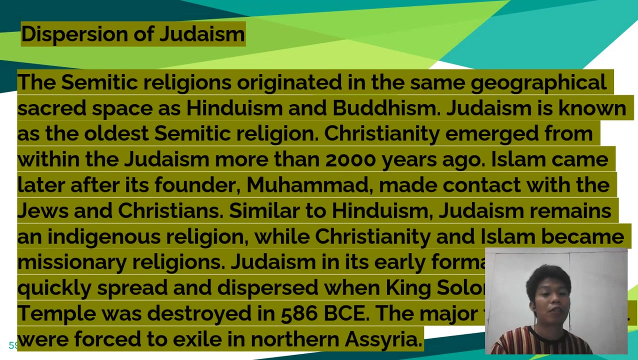 Hinduism and Buddhism were also practiced. For example, in Thailand. they practiced Hinduism. Buddhism was also practiced in China. Dispersion of Judaism. The Semitic religions originated in the same geographical sacred space as Hinduism and Buddhism. Judaism is known as the oldest Semitic religion. 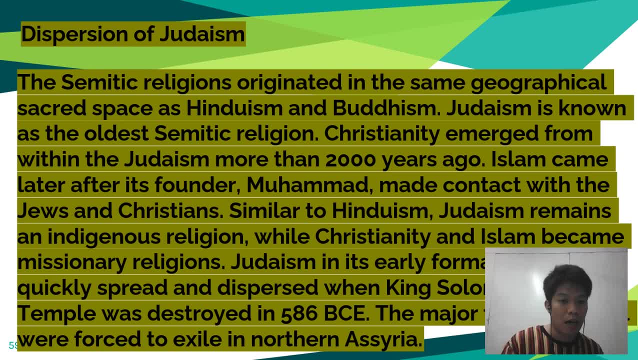 When we say Semitic religion, it is called as that because the forefather of Jewish or Hebrew people was one of the sons of Noah It's Shen. That's why it's called Semitic religion. Christianity emerged from within the Judaism more than 2000 years ago. 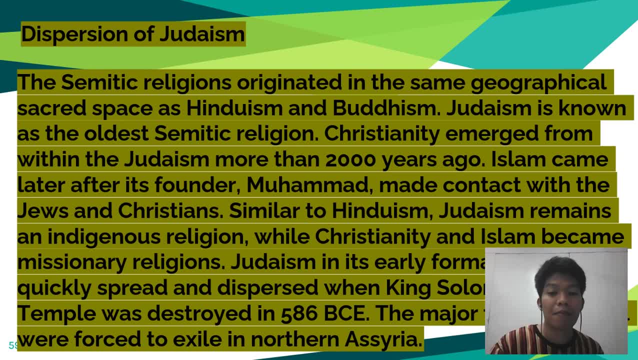 Islam came later, after its founder Muhammad made contact with the Jews and Christians. Similar to Hinduism, Judaism remains an indigenous religion, while Christianity and Islam became visionary religions. So that's the difference between Judaism and Christianity and Islam. 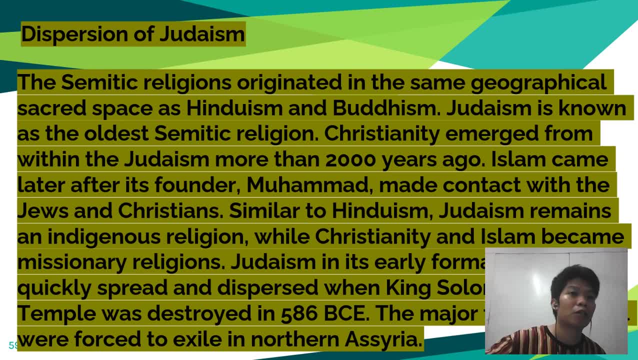 because Judaism, they are not aggressive in terms of spreading their religion because mostly Judaism is only practiced by Jewish people, by the Jews. While Christianity and Islam are spread out to other people through other races, Judaism, in its early formative years, quickly spread and dispersed. 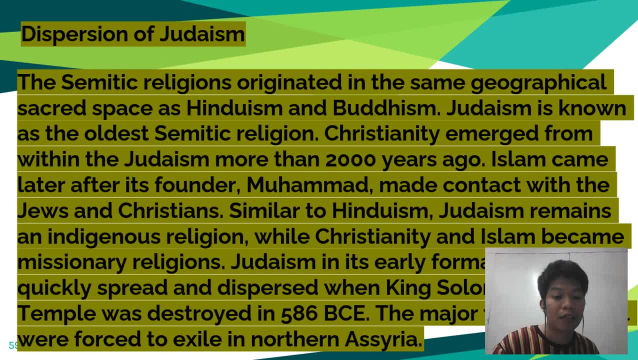 when King Solomon's Holy Temple was destroyed in 586 BC, Major tribes of Israel were forced to exile in northern Assyria. So it is. If you read the Bible in the Old Testament, you will learn that every time the Israel was being conquered by other nations. 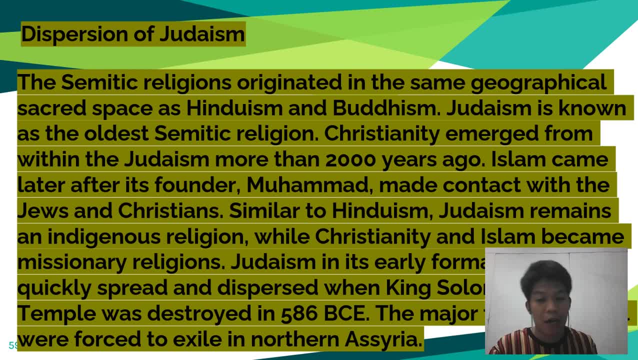 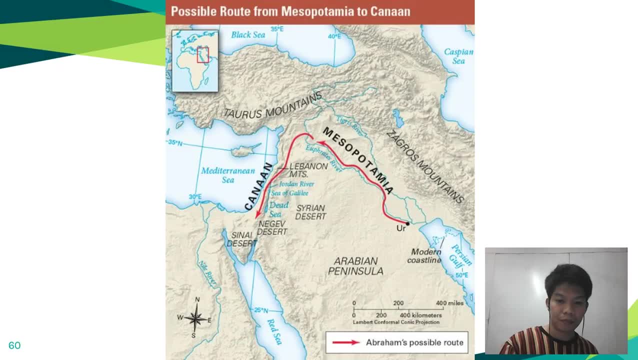 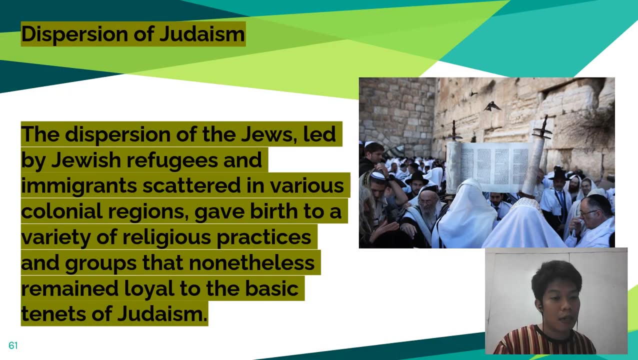 people, or the Hebrew people, spread out to other places such as this case: Dispersion of Judaism, Dispersion of the Jews, led by Jews refugees and immigrants gathered in Paris called Norwiches, gave birth to a variety of religious practices. 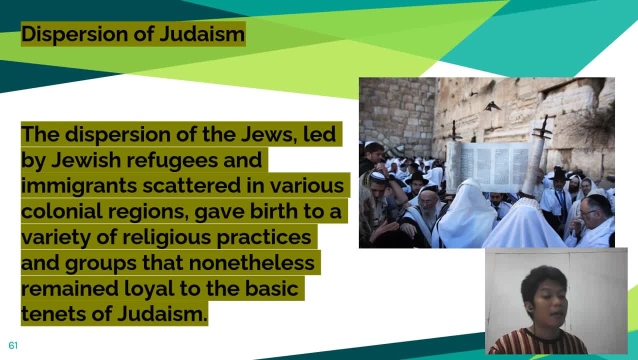 and groups that nonetheless remained loyal to the basic tenets of Judaism. That's what I've said. Israel was conquered by other nations for countless of times. It was in 1948. it was. it was conducted in the United Nations. 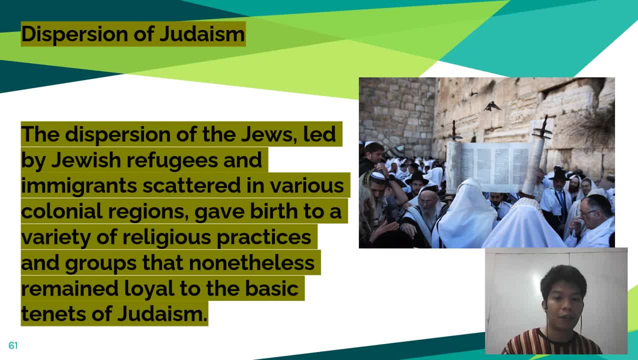 and regarded Israel as the nation of Israel, as the independent state of the Israeli people. It was 1948 when they went back to their original land, But during the times when they were scattered around the globe, although until today there are still Jewish people. 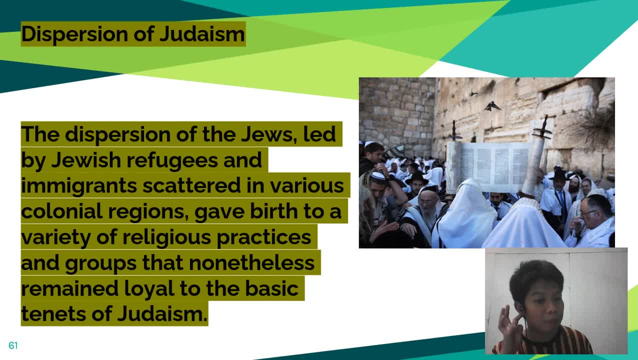 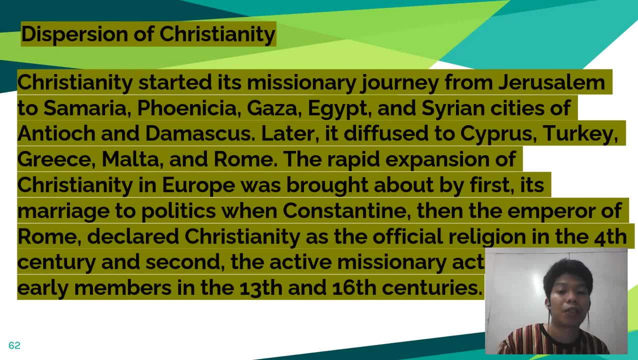 around the globe scattered, they still practice their religion with them. Dispersion of Christianity. Christianity started its missionary journey from Jerusalem to Samaria, Phoenicia, Gaza, Egypt and Syrian cities, and Shogunate, Damascus. 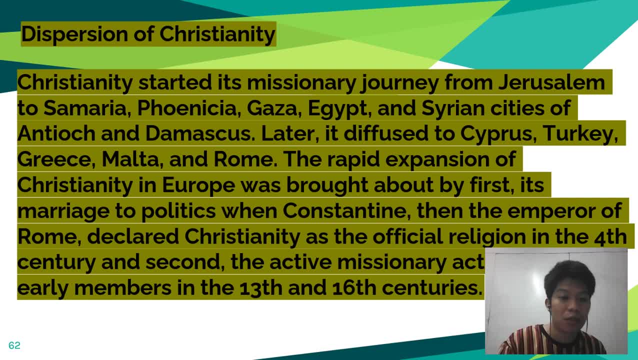 Later this year it refused to Cyprus, Turkey, Greece, Malta and Rome. The rapid expansion of Christianity in Europe was brought about by, first, its marriage to politics with Constantine. Constantine, the emperor of Rome, declared Christianity as the official religion in the world. 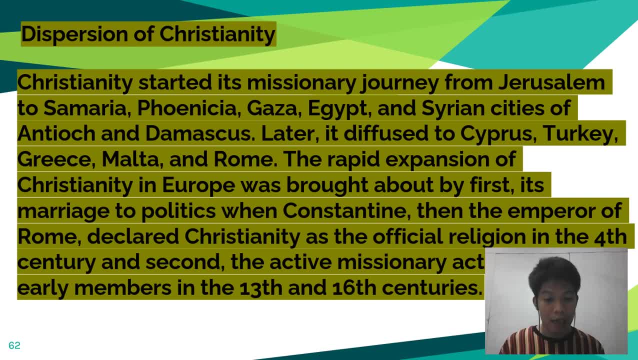 In the 4th century, the active missionary activities of the early members in the 13th and 16th centuries. If you study the New Testament and the early events after the death of Christ, you will learn the dispersion of Christianity. 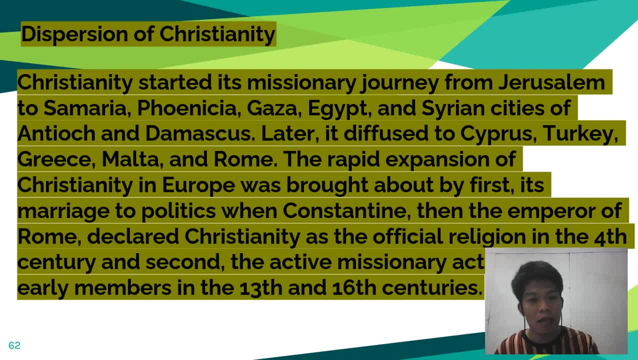 from Israel to other parts of Asia and Europe. Because Emperor Constantine accepted Christianity, he merged it to their original religion, which is Mithraism. So he combined Christianity and Mithraism, he combined the religious beliefs of both religions. 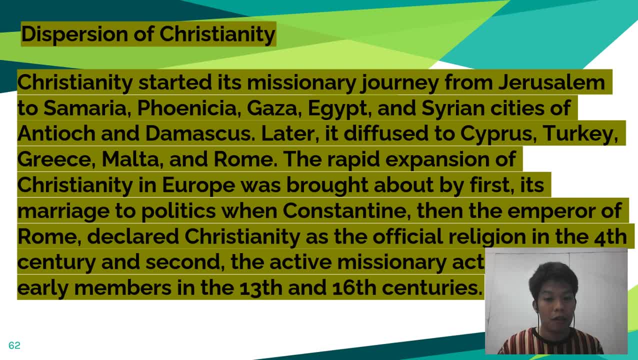 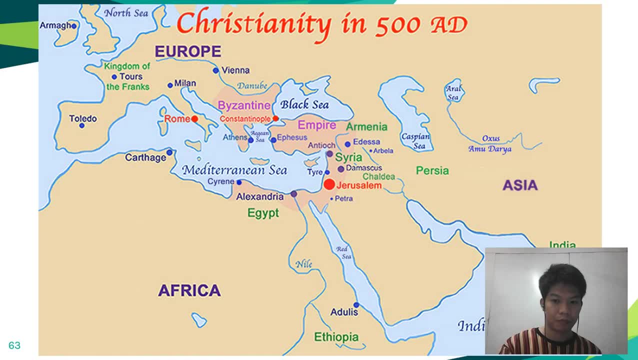 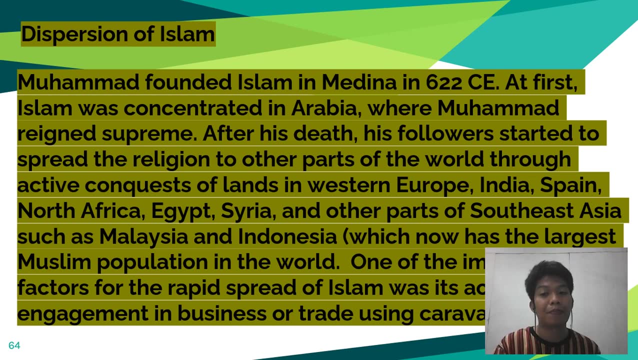 and they spread out this religion in the Europe. The dispersion of Islam. Muhammad founded Islam in Medina in 622 CE. At first, Islam was concentrated in Arabia, where Muhammad ran supreme. After his death, his followers started to spread the religion. 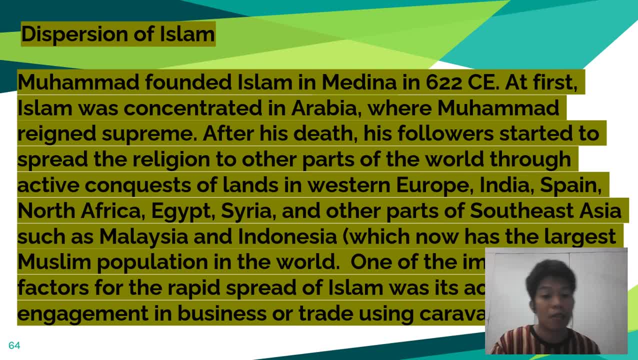 to other parts of the world through active conquest of lands in Western Europe, India, Spain, North Africa, Egypt, Syria and other parts of Southeast Asia, such as Malaysia and Indonesia, which now has the largest Muslim population in the world. 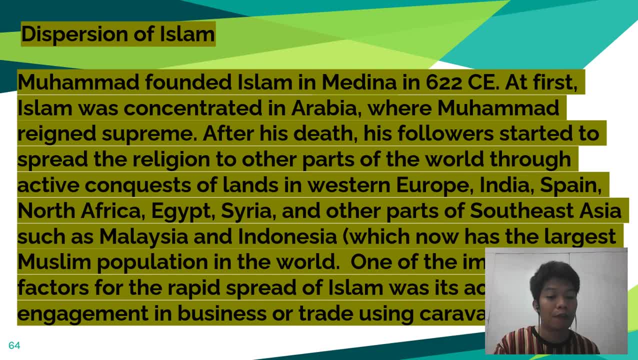 One of the important factors for the rapid spread of Islam was its active engagement in business and trade using carpentry. We discussed earlier that one of the tools used by Islam in order to spread out their religion. 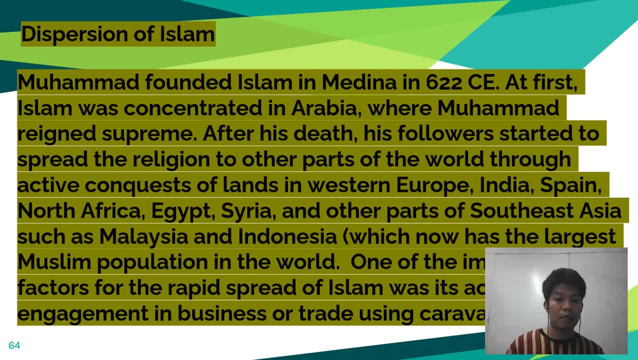 is through business and trade, But there were instances in the past that they engaged in crusades wherein they influenced other people from other countries through wars. That's what they called the holy war. 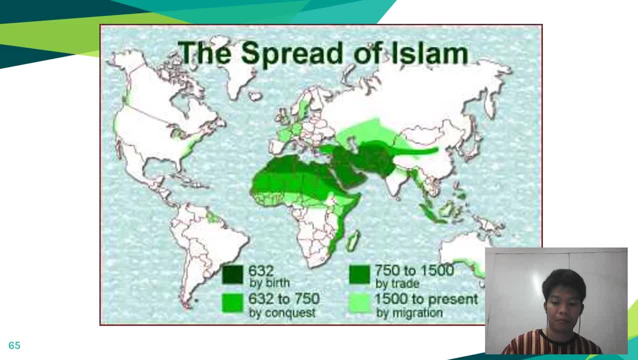 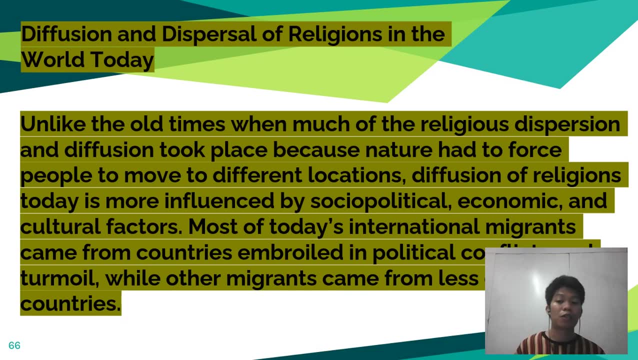 or the jihad, Deficient and dispersal of religions in the world today, Unlike the old times, when much of the religious dispersion and deficiency took place because nature had to force people to move to different locations,